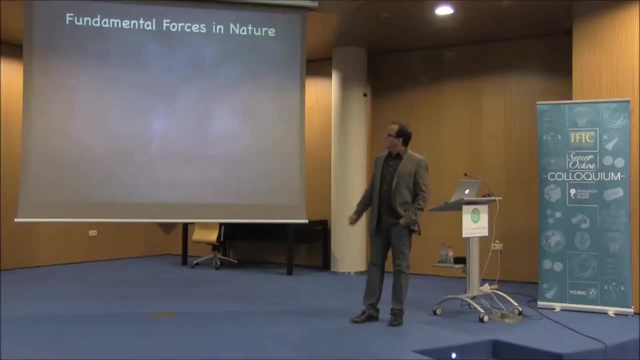 fundamental forces. no, We have gravity, we have electromagnetic force, we have the weak force, we have the strong force and five years ago we discovered a new force, okay, Which is the Higgs force. Then if you have, let's say, two quarks, they can interchange, gravitons, they can interchange. 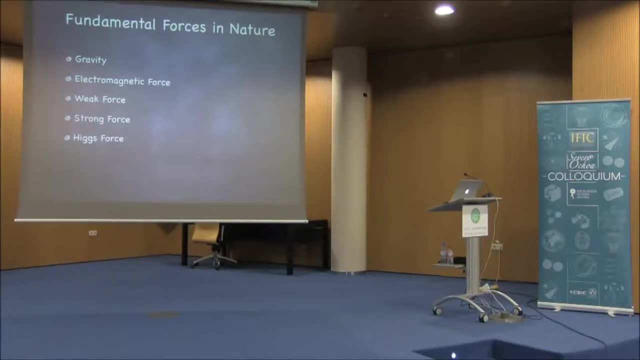 a Z, a photon or a gloom and a Higgs, And then in this way we could understand the interaction between matter. okay, Actually, we are lucky that now we have a new force in nature. Maybe soon the LHC will discover something more. no, 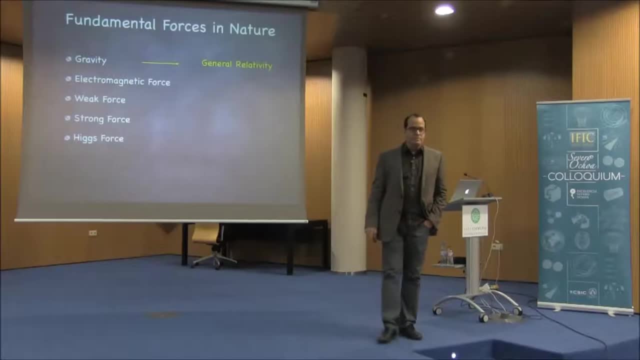 Gravity can be described pretty well with GR. okay, So far you can do pretty well And the standard model can do pretty well. for the rest, okay. When I say pretty well, it's that you can explain most of the properties okay. 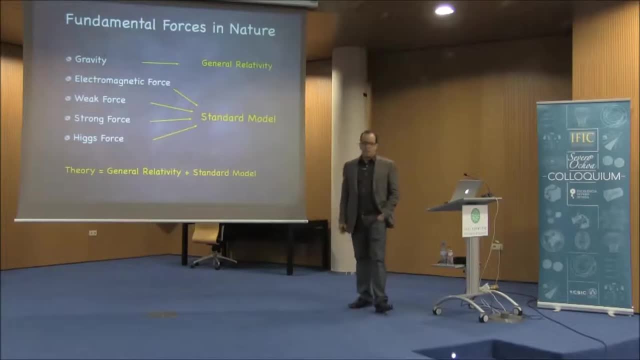 And it is easy to say that. you can say that the theory of fundamental interaction today is just GR plus a standard model. okay, When these two theories together, you can do pretty, pretty well. okay, You can describe most of the properties that we see today. okay, 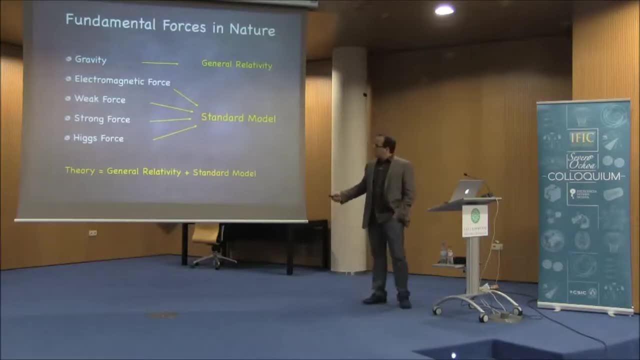 This is what we see in nature. okay, Beautiful to see that the standard model of particle physics can do the job for four. okay, And you always can make a joke to gravity people that you know you do. particle physics, you do more than a thing. 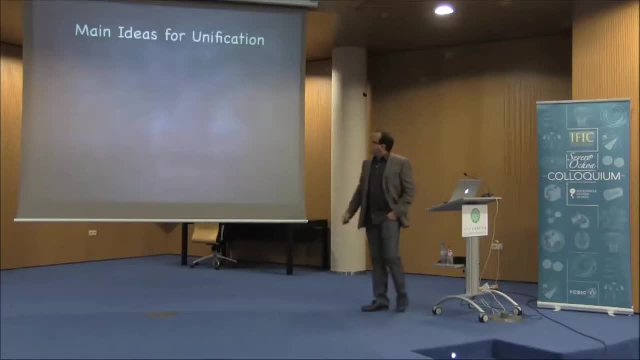 This is not true? okay, Now the people for many, many years tried to study the unification forces, And the main idea behind that is that you try to build a theory which could be way simpler than the standard model of GR and try to put everything together. 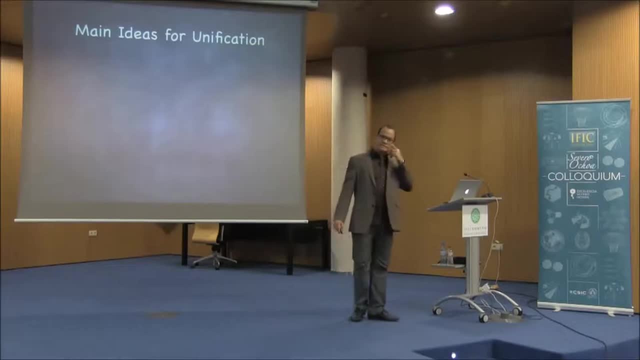 to see how you can simplify. okay, This is the key idea of unification: simplicity. okay, We don't know if this is true, but the people tried for years. okay, Then one idea that has been in the market for a long time. 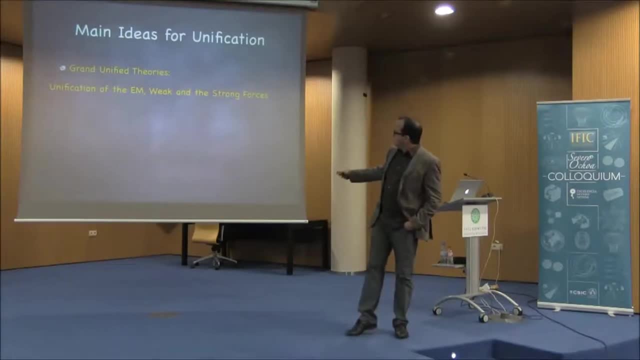 is the idea of GR theory. In that context, you can unify the electromagnetic, the weak and the strong interactions. okay, I will discuss mainly these things. There are other ideas which are way more speculative. okay, For example, you can maybe understand the unification. 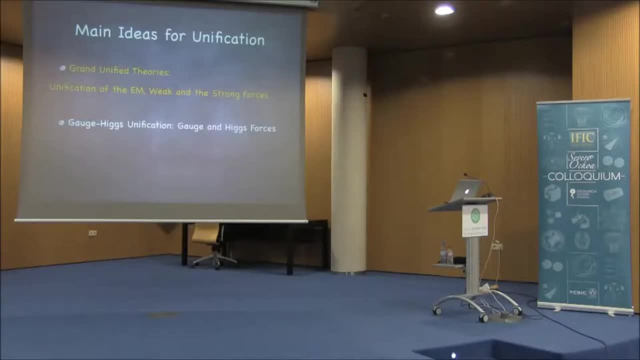 of gauge forces and the heat force in so-called gauge-heat unification scenarios. They don't work so well. People try, Of course. you heard that there is something called string theory or something. Sometimes, you know, people call this in different ways. 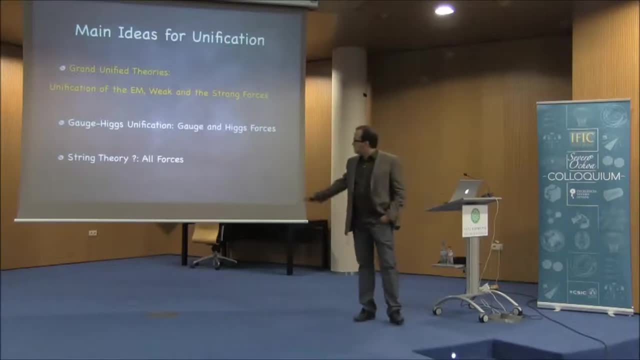 The main goal is to unify everything. okay, But these are really even way more speculative than this grand unified theory because, at least for people working in particle physics, we understand pretty well the standard model of particle physics. We know how to use quantum field theory. 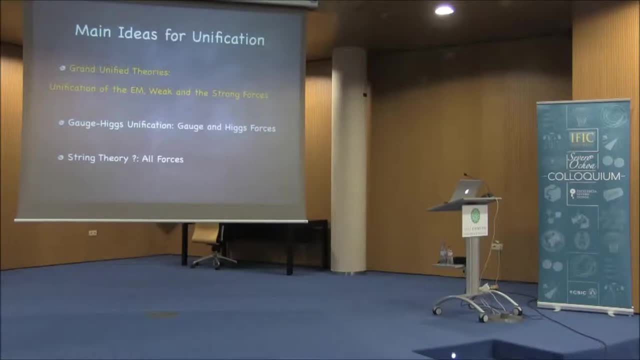 And in grand unified theory you face the issue that the theories are even simpler than the standard model and you can use all the tools of quantum field theory to study all the predictions, But once you go beyond, in my opinion it's quite complicated. 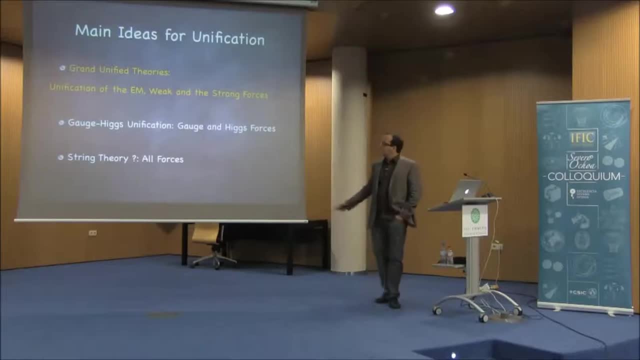 That's why I will focus mainly on that And I will try to explain all these properties. Now let me start with this story about unification In 1974, before I was born- George I from Harvard, Helen Quinn from Stanford and Steve Weinberg. 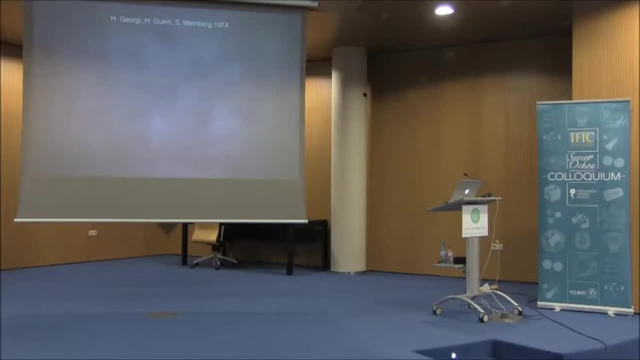 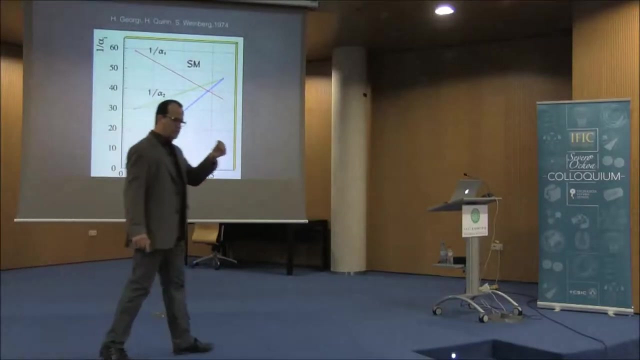 at that time he was at Harvard. they wrote a very interesting paper where they basically did the following: This alpha, alpha 1, alpha 2, alpha 3, these are basically a parameter that can give you an idea how the matter, for example, 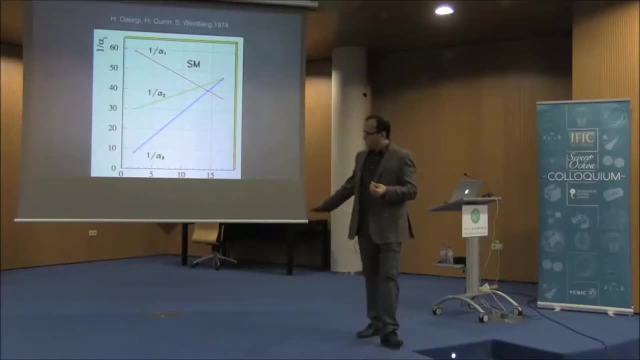 feels given interaction. Like: alpha 3 tells you, for example, how the quarks feel the strong interaction, how the plumes between each other feel the strong interaction. And alpha 2 and alpha 1, together they can describe the weak and the electromagnetic interaction. 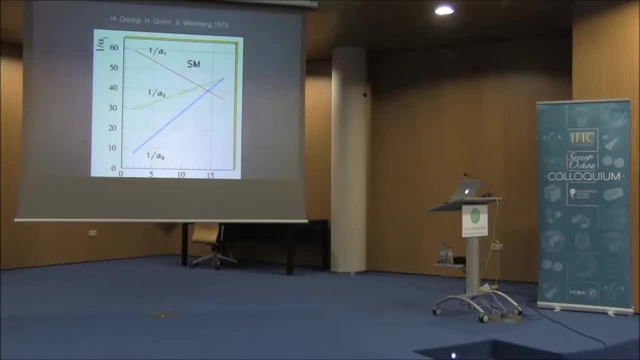 And they did an interesting exercise where they studied the evolution of the couplings with the energy scale And they found that somehow they tried to get together In 1974, they didn't really knew these values here that you see, And then I will give all the credit to them. 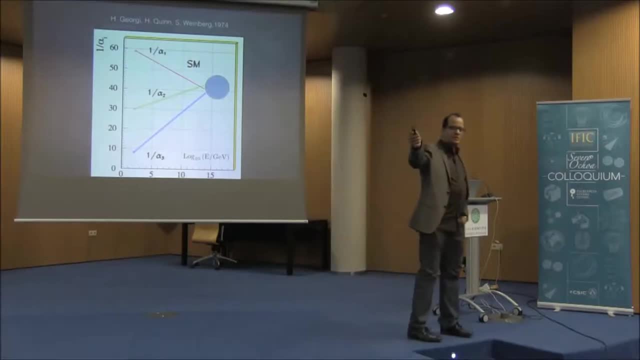 They saw something there that maybe these gauge couplings could, some energy scale, have the same numerical value, And maybe you could say, maybe this is an accident, no, But this is a little bit profound. okay, Because today, for example, 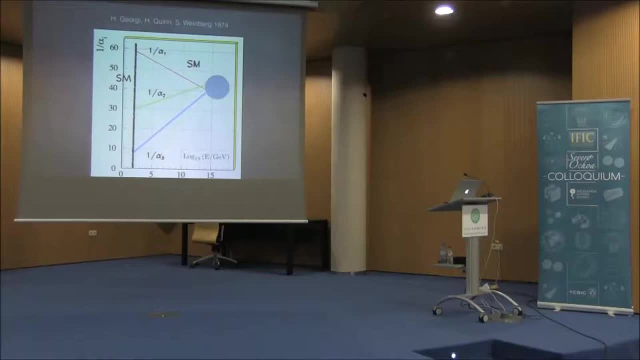 we know that below, let's say, the electric wheel scale, we have the standard model that can describe physics very, very well. We have the Large Hadron Collider exploring this region of the parameter space, the Tb scale. okay, And if this is true, 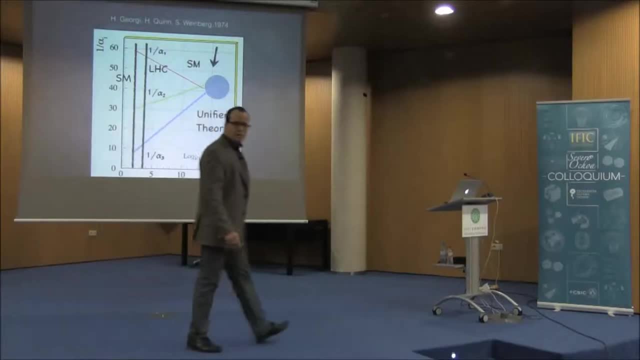 at some energy scale, you can expect a new symmetry or a new theory that we call unified theory, because all these interactions behave in the same way. Okay, But the interesting part here is that for years and years, experimentalists built many good experiments. 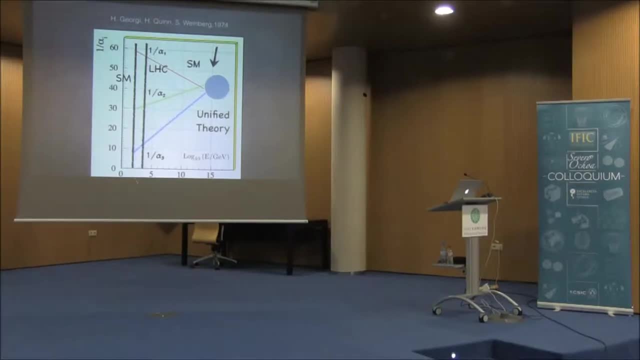 And so far, the best that we have is the Large Hadron Collider exploring the Tb scale, And there is no really hope to build any collider that can prove a super high scale. okay, And then the first thing that I want to say is that 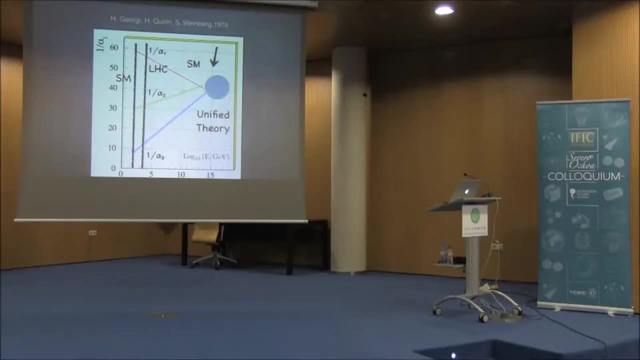 maybe this is very beautiful, but there is no way to know about this in a real experiment. Okay, Yes, Because you cannot produce the new fields that maybe live in this grand unified theory at a high scale. Okay, But maybe this is true, okay. 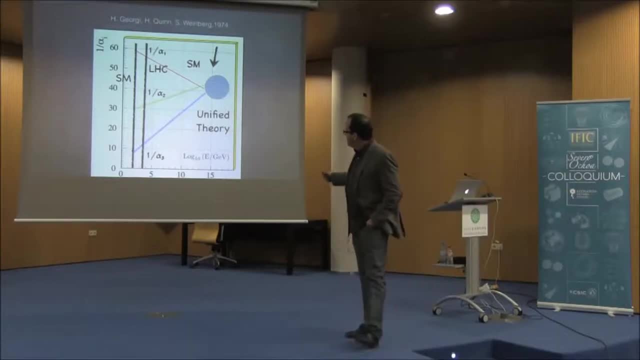 And we have to think about that. But keep in mind, it would be great if- this you know, accidental, or if you can explain- unification could be realized at the lower scale. And I will tell you why. typically, this is very, very hard. 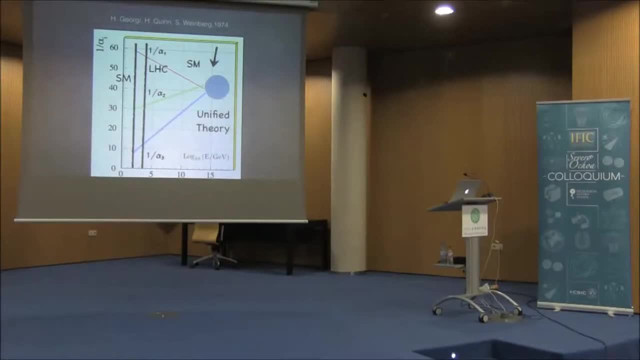 Okay, And this is a simple idea of grand unified theory from the bottom-up approach. You use the information that you have at low energy, you try to extrapolate your theory at high scales and maybe you try to learn what could happen. Okay. 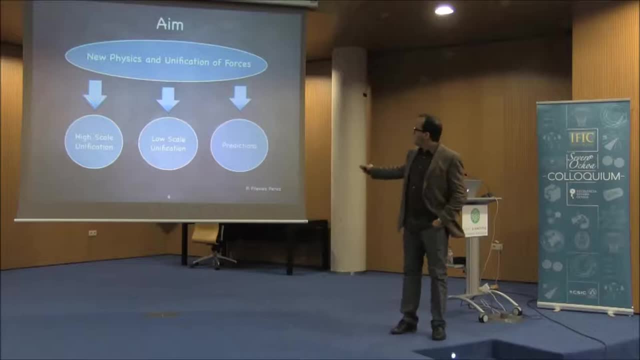 Now what I will do in this colloquium is I will talk about different ideas for new features. on the unification, I will focus on the main scenario, that is, the high scale unification, where you cannot really test this in a collider but you have predictions that you can maybe look for. 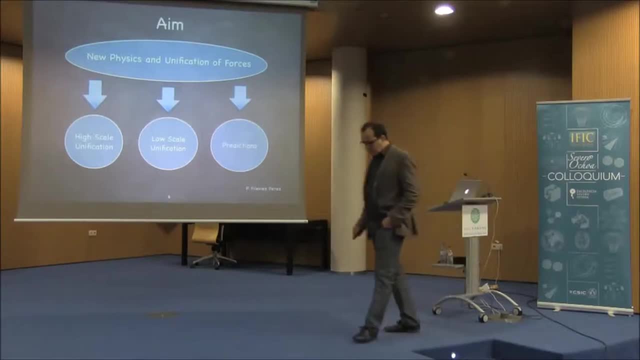 And I will try to tell you a different approach that tells you that maybe there is a way to unify a very low scale and you maybe can hope to test this in colliders. Okay, That would be really fantastic. Okay, And I will talk about all the predictions. 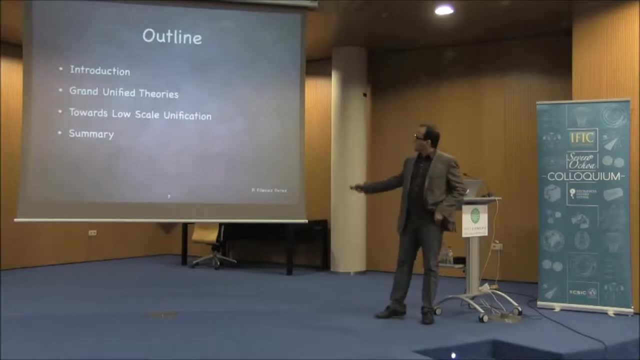 in different scenarios. Okay, Now this is the plan Introduction for students. I will talk about grand unified theories, I will tell you how to unify or how you should follow, which idea you should follow to unify the low scale, And I will give a summary, which is: 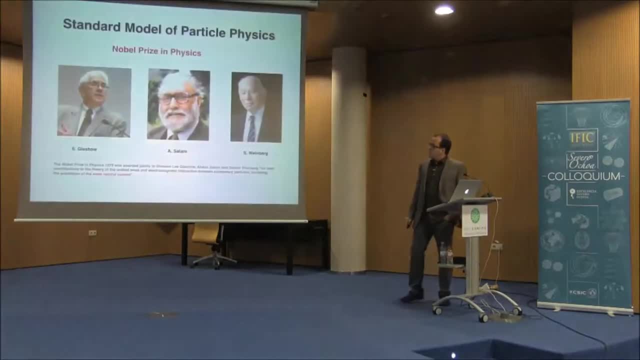 maybe you can keep after this talk. Introduction: Thanks to Glashow Salan and Steve Weinberg, we have this amazing theory for the so-called standard model to describe the electroweak, the electromagnetic and the strong interaction. 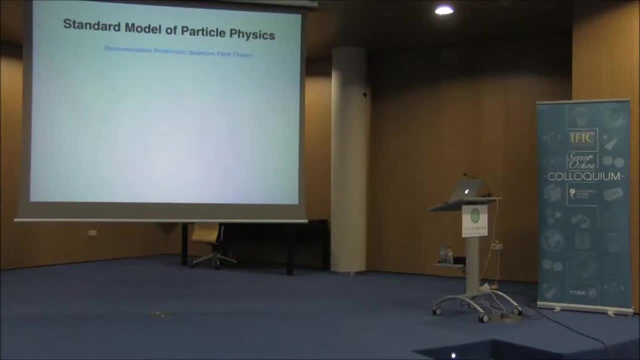 Okay, This is a randomizer. relativistic quantum field theory based on this group: SU for strong interaction, SU and U to describe the electroweak and the electromagnetic interaction. For each group. you have a gauge coupling This alpha dimension before is. 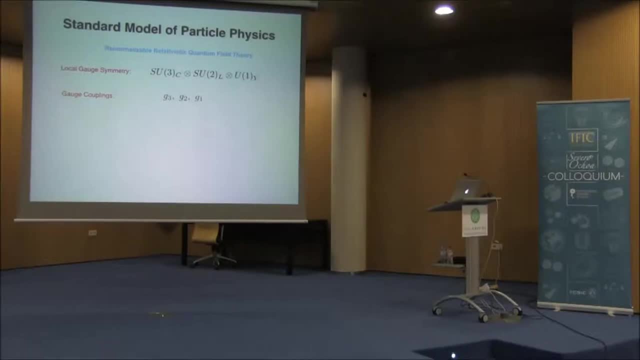 just G squared divided by 4 pi. just the same, just a different way to write. And in this way you can. if you study the values of these couplings associated to different interactions, you understand how matter feels to different interactions, and so on. 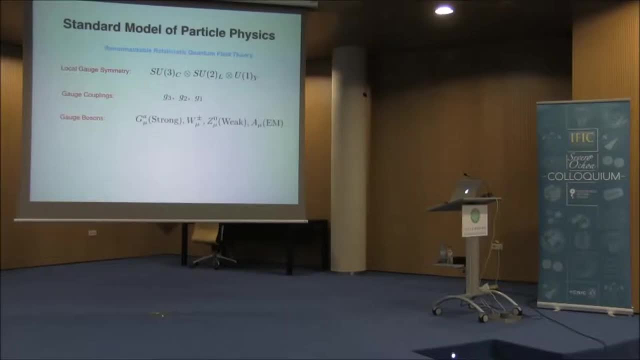 And in the standard model we have the physical fields: the gluons for strong interaction, the W and the C for the weak interaction and the photons for the electromagnetic interaction. Okay, We have quarks and leptons. Okay, They have different properties. 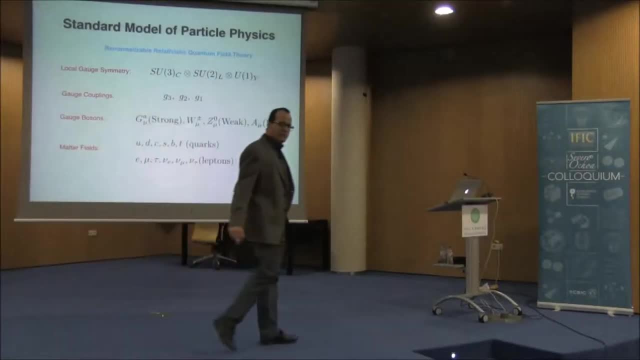 The quarks, they feel the strong interaction. The leptons: they only feel the weak and the electromagnetic interaction- some things They have. in 2012, we were lucky to because the LHC managed to discover the Brown and Blair-Hicks boson. 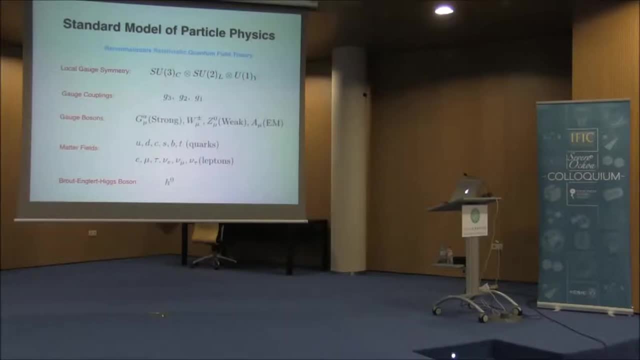 and now we know that all these fields here, they have a spin one. These fields, they have a spin one-half and this is the only one in the theory that has a spin zero but was always crucial in the theory, as I will explain later. 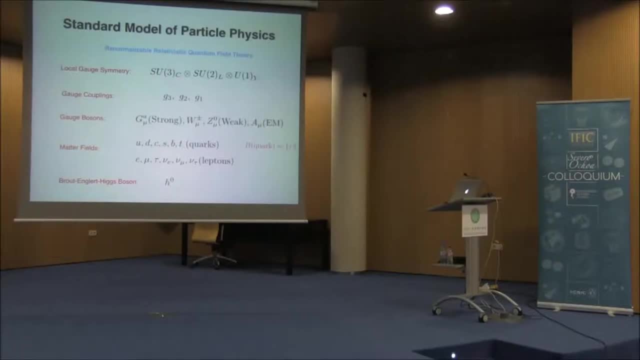 The quarks. they have an interesting property is that they have a quantum number that is called barrier number. They have barrier number one-third. A proton is made of three quarks. The proton has barrier number one And the leptons. 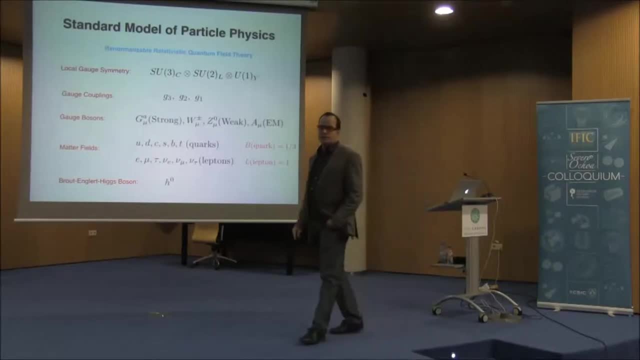 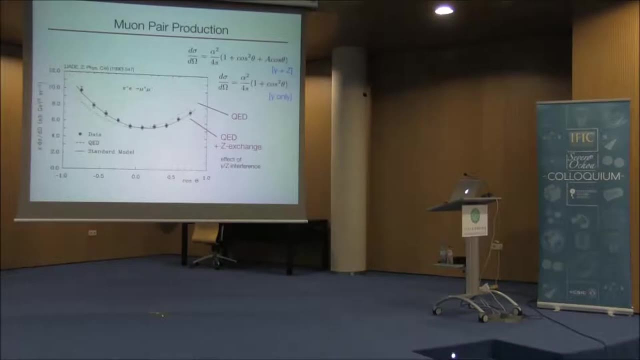 they have a different quantum number that is called lepton number. that is one for all the leptons. Okay Now the standard model has been doing pretty well for a long time. This is a plot from you know, pretty old plot from 1990,. 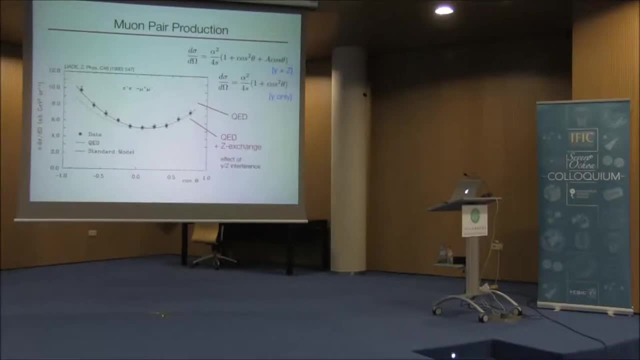 where the people compute the E plus and minus collision to mu plus, mu minus and you can see that if you try to match experimental prediction using only QED you cannot do the job. but once you put the Z you can actually explain very well the experiment. 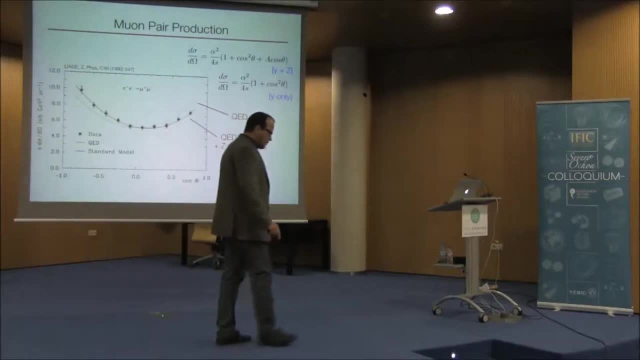 in very, very high precision. Okay, Already, for a long time we knew this set of the standard model was doing very, very well. Then this is why we call the standard model a theory of nature. no, This is a collation of many, many, many studies. 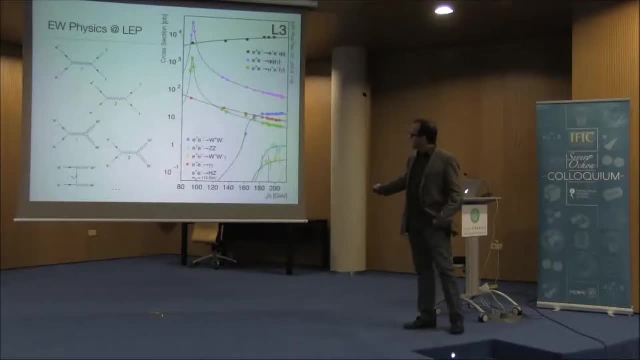 at the lab colliders. When you study many, many, many cross-sections, you do again the theoretical calculation. check the experiment and you can see that you can be in agreement with all. most of this experiment very, very, very well. no. 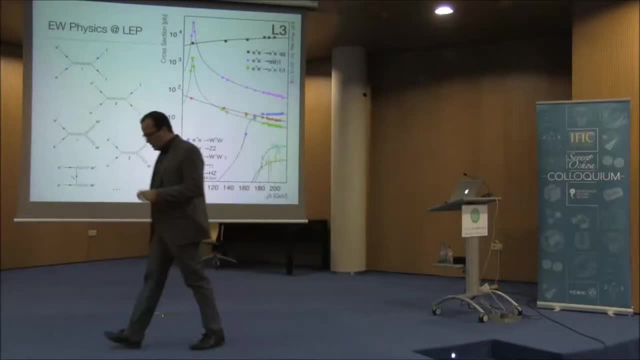 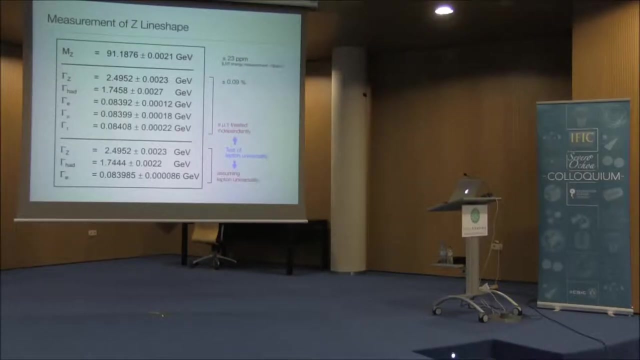 This is actually pretty, pretty impressive. The standard model is the best theory that we have in nature to explain many experiments with high, high precision. okay, I just will give you one idea how well we know these things like the mass of the Z. 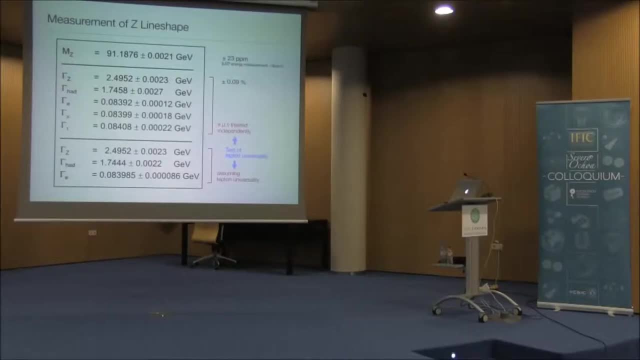 We know these things in super high precision: the decays and so on. This is so good that it's hard to imagine that you can do better than any other theory. okay, Now, for a long time we knew that we could explain. 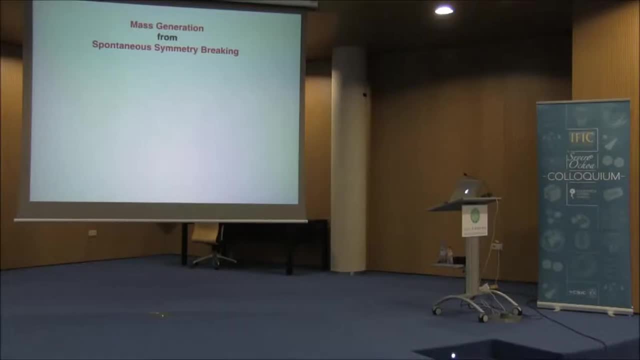 many properties from the standard model, but we had no idea how to explain the mass generation of the standard model And the hypothesis was that you have this symmetry and we use the spontaneous symmetry breaking, because this is the most predictive way to understand generation of masses. 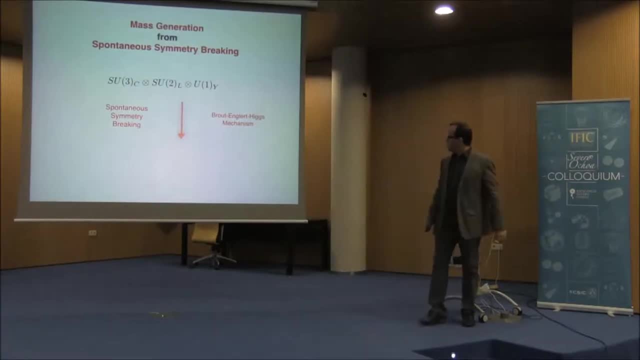 and this was postulated by the so-called Brown and Glare-Hicks mechanism where, using this mechanism, we used to break, we used to assume that this symmetry, the electroweak symmetry, was broken to U1, electromagnetic, and this way explained. 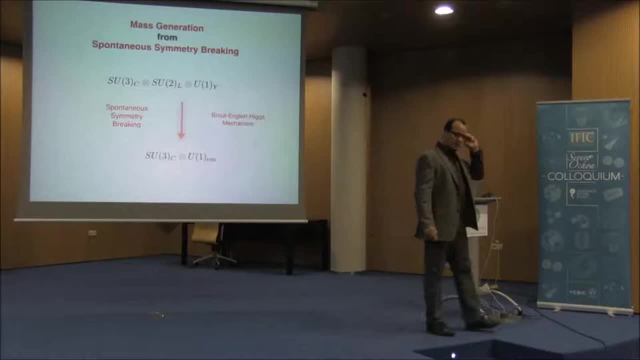 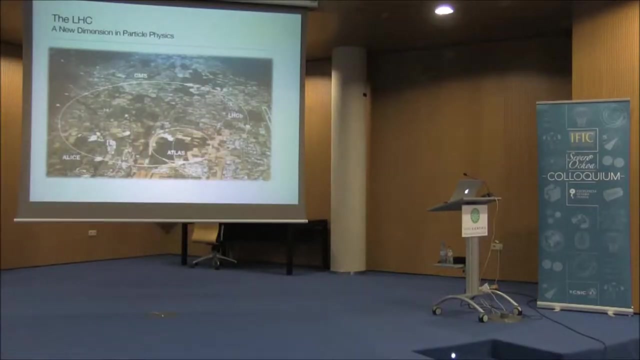 why the W and the Z were massive and the photon is massless as well. okay, And as you probably most of you know, this is the Nobel Prize of 2013,. okay, Now, thanks to this great experiment, the Large Hadron Collider. 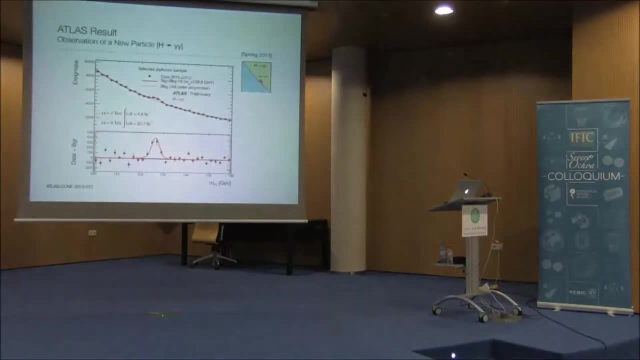 thanks to CMS and ATLAS, now we know that the Higgs is a real thing. okay, This is the plot where you discovered the Higgs to gamma-gamma, and now we know this is a real thing. we know pretty well now. 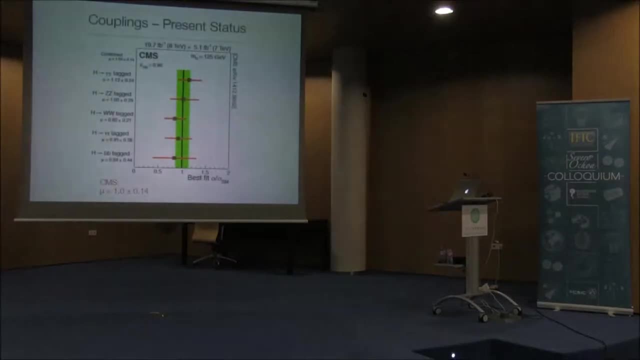 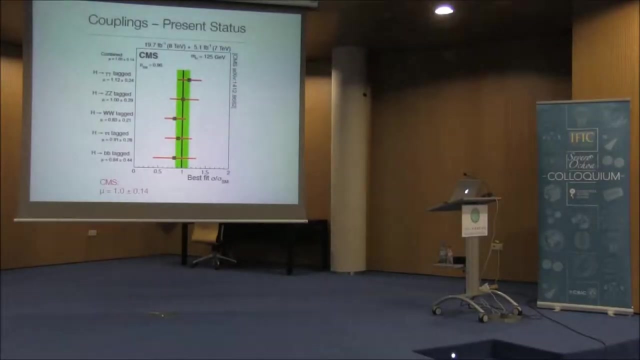 the properties of the Higgs. still, these are basically how the Higgs decay to two-fold. okay, If you compare to the prediction in the standard model and the prediction that you, the measure that you have in the experiment, you can see that in many of the channels. 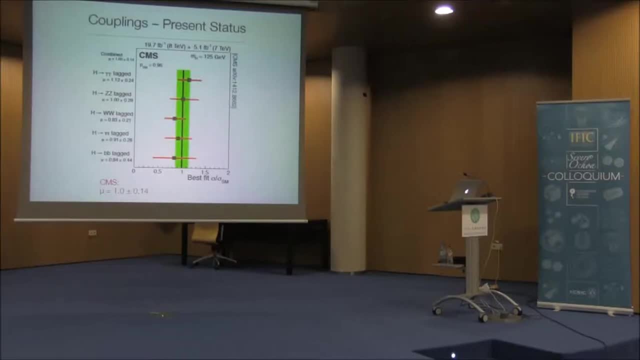 the Higgs can decay to all the gauge bosons. these are virtual W and the Z and some of the electrons and quarks and today we know very well most of the properties, not all of them, but we know very well no. 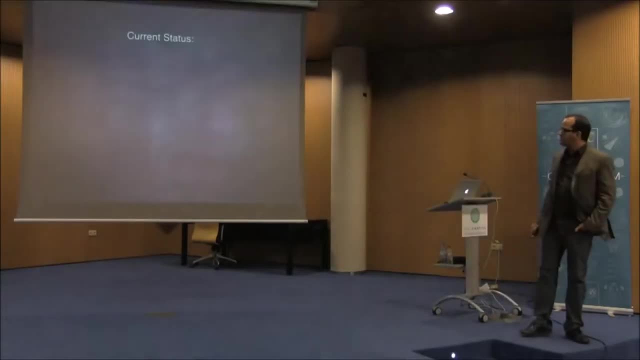 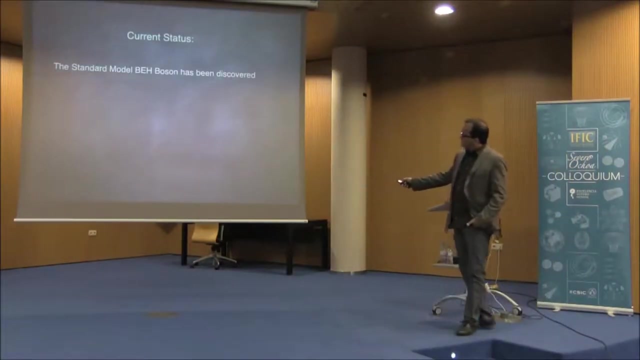 But somehow this is actually closing a chapter in particle physics. okay, Basically we can say: the standard model Higgs. now we know that it's a real thing. it's a particle. when you spin zero and you have really the spontaneous breaking. 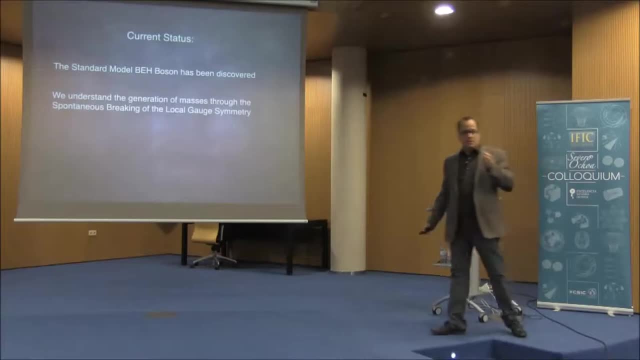 of the symmetry to generate masses. this is the fundamental way to understand the generation of masses in nature. okay, And it is important to say that the standard model provides a good explanation for most of the experimental results that we have in particle physics. okay, 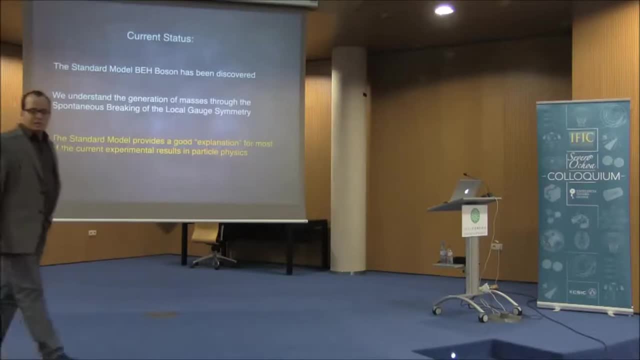 And then this is the only thing that we know. that is true today. the rest of all the ideas that you see in the market, they are just speculations, ideas, fantasies, any idea. we have no idea. okay, The standard model of particle physics plus GR. 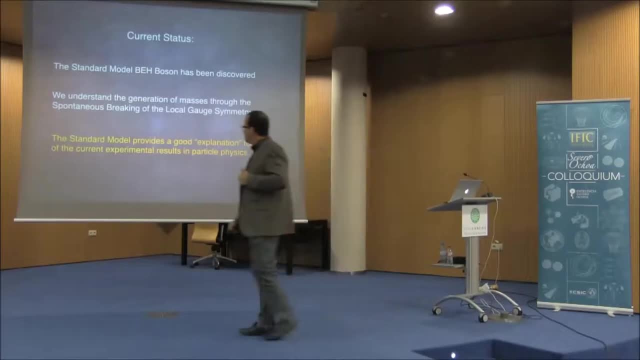 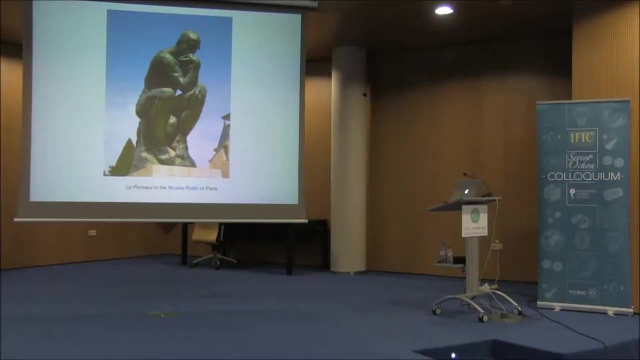 in this you do very, very well. Okay Now, even if the people have been thinking for a long time, it's good to think hard again. because why again? Because now we know that the Higgs is there. before we were not sure. 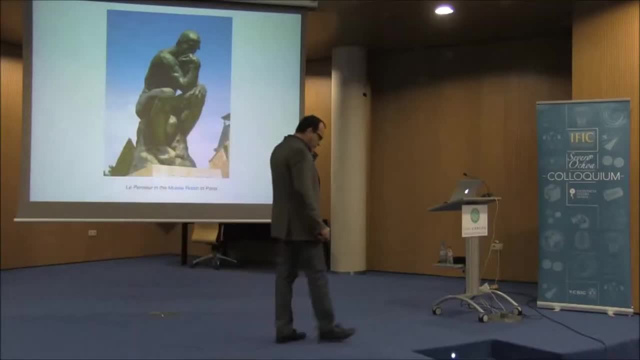 maybe the symmetry was working in different ways, but actually the Higgs is a real thing. spontaneous symmetry breaking is playing a role in nature and it's time to think even harder now. Okay, Now of course you can say: 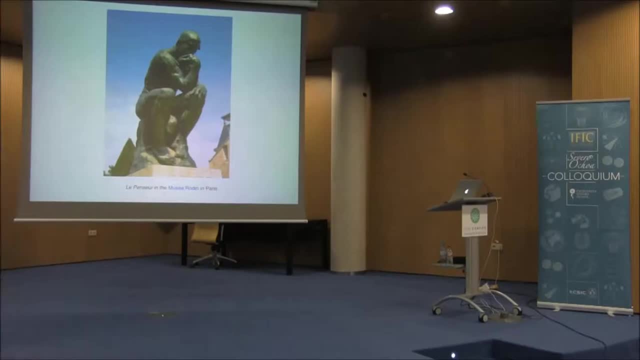 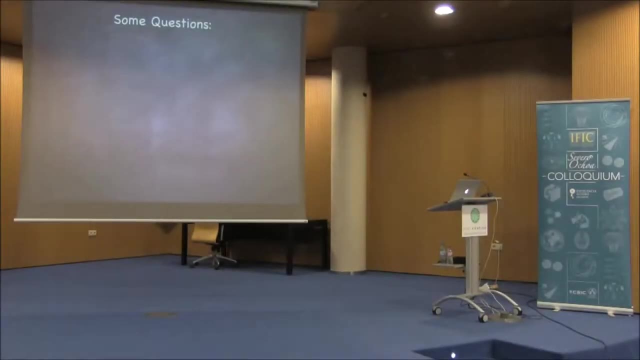 I'm thinking different places. Paris is a good place to think, especially if the weather is good, and I will just talk about some questions that you can ask. Okay, One of the questions that you can ask is why the standard model interactions are so different. 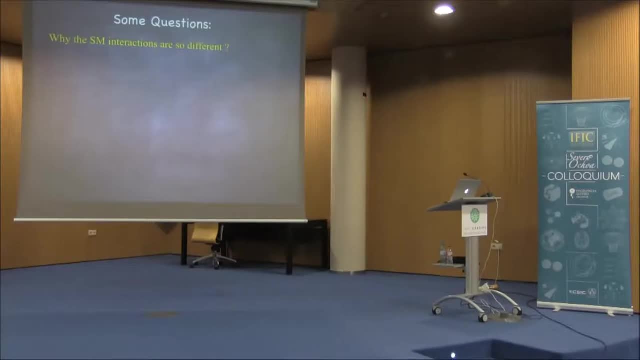 You have the strong, the weak and the electromagnetic interactions and they are very different. These values of the parameters, they actually have different values and they matter in different ways. these interactions, We have no idea if you try to explain the masses of fermions. the electron mass is so tiny and the core masses, like the top mass, is so large that we have no idea. Today we know that the neutrino, for example, is massive. This is a good question to think about, and the standard model doesn't provide a mechanism for that. 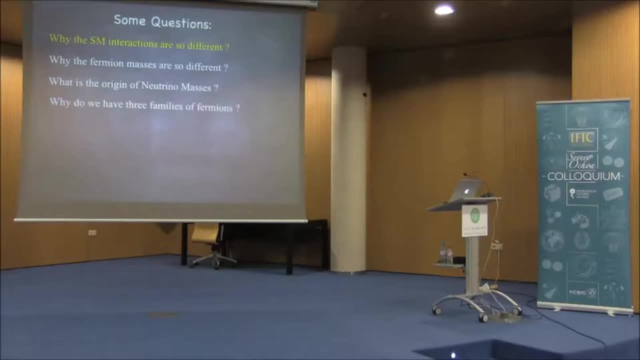 This is a good thing to think about. physically, on the standard model, We know that we have three-family fermions, but we have no clue. why is that? Today, after the Higgs discovery, this equation is even more relevant, because it used to be that we were allowed to put the four families 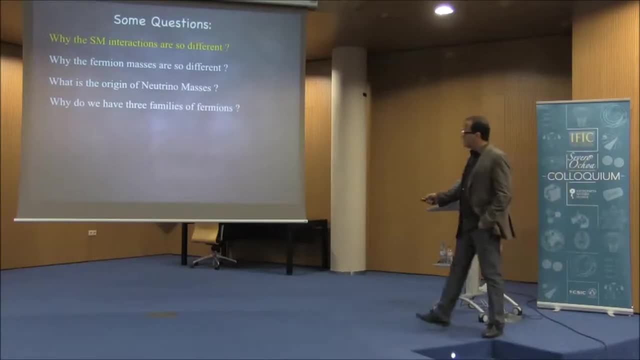 even properties, higher families. but this today is not possible in any model, physically, on the standard model, because this will destroy the property of the Higgs boson. You cannot do that anymore. I would say this question is becoming even more interesting today. 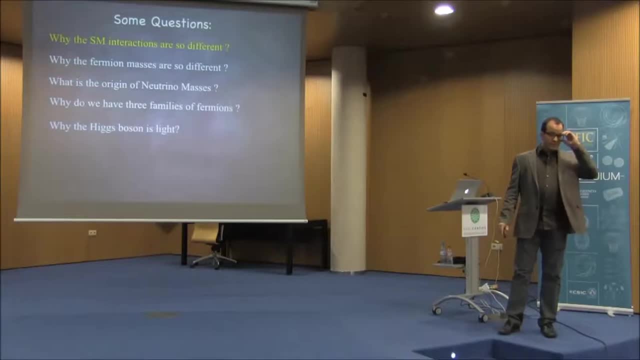 And the Higgs mass was discovered with mass of 125 Gb. We have no idea. why is that? Nobody knows. Okay, This is a very interesting question And if you go, of course, to cosmology, we know that there is cold and matter in the universe. 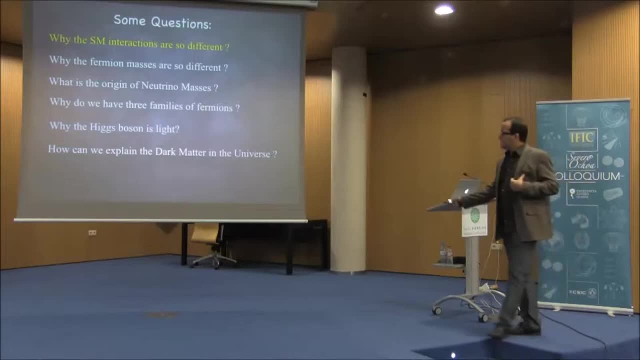 We think that there is cold and matter in the universe. The standard model doesn't provide a mechanism for that. It would be nice to have, And at the same time we call us matter, and since we don't see our anti-matter guys around, 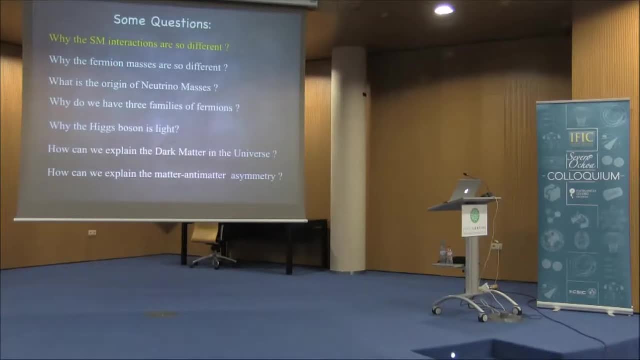 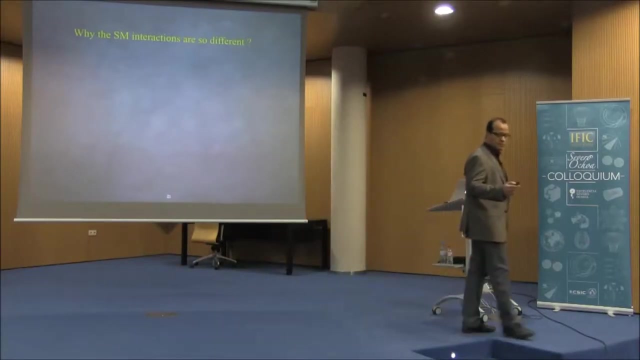 it's important to understand why we are around and they are not around, And then, typically, the standard model cannot really explain this big difference. Okay, Now I will focus in this colloquium mainly on this question here, Why the standard model interactions are so different. 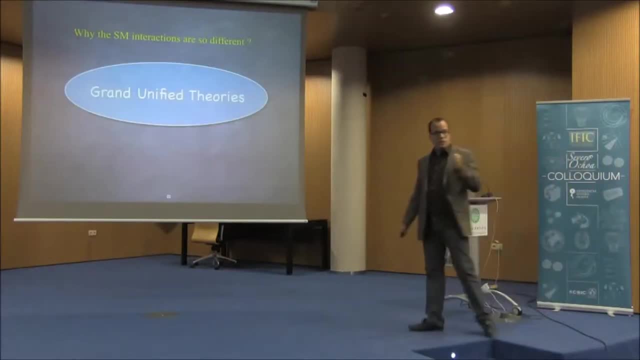 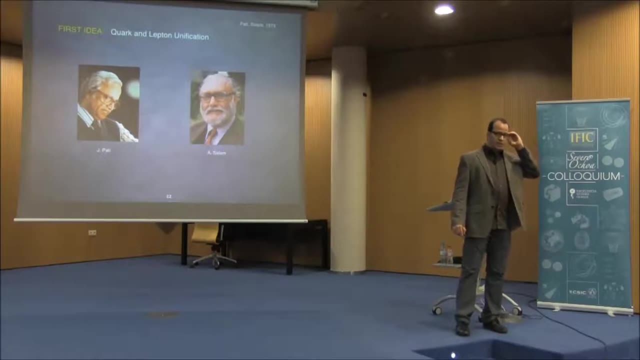 Okay, The main. the best way to explain that is using Grand Unified Theory. Okay, The first idea in the main theory in the market to think about Grand Unified Theory was actually pointed out by Yogesh Pati and Andous Salam. 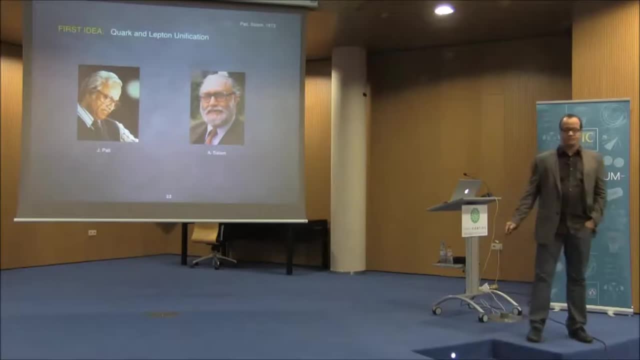 the same Salam from the standard model. Great physicists? Okay, They basically. according to Yogesh, he was at ICDP in Trieste. you know, bothering Salam. How is it possible we have quartz and lepton? What is that? 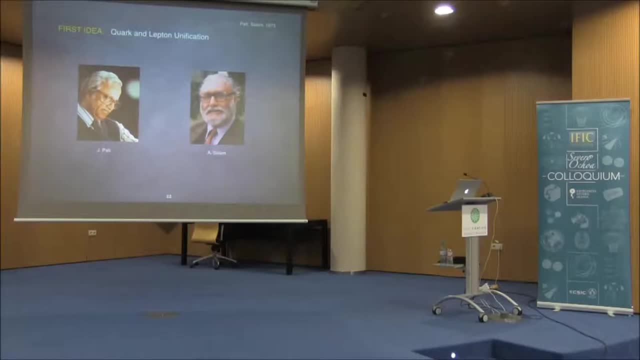 Why matter has to be different, Why they cannot be the same somehow, And they proposed the so-called idea of quartz-lepton unification, which generically predicted. a very interesting phenomenon is that I told you, in the standard model, that quartz they have. 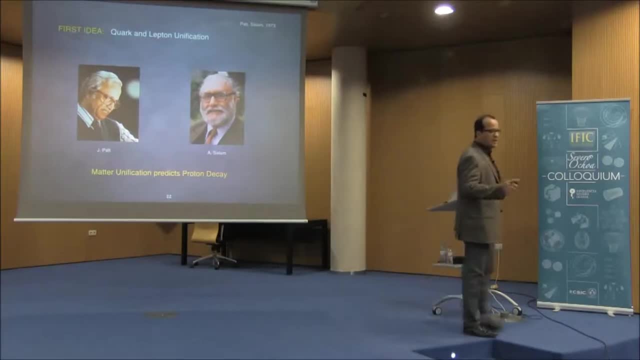 barren number. This symmetry is actually accidental symmetry. in the standard model It's broken at the non-perturbative level, but it's basically pretty good symmetry. And in the standard model you know that the proton is actually stable because 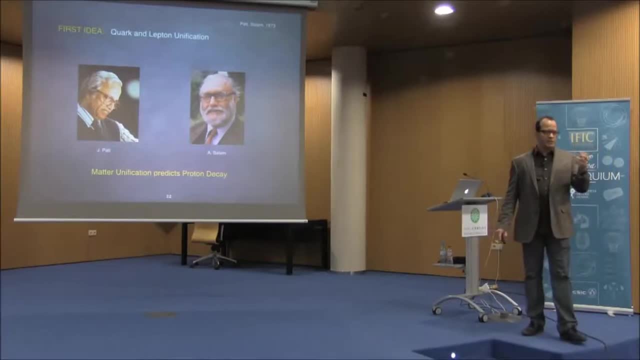 even the barren number is broken in three units in the standard model. To get proton decay you have to break it in one unit. Therefore, this is a very hard prediction of the standard model of particle physics that proton is stable. Okay. 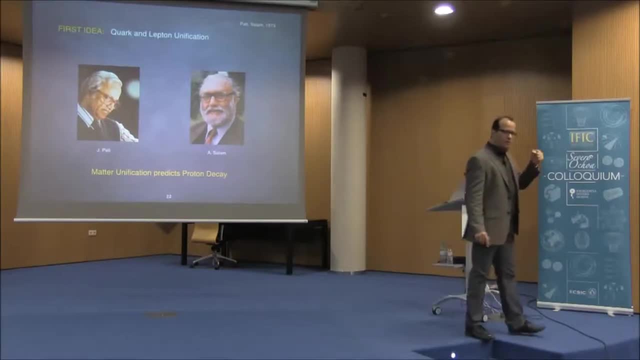 Even at non-perturbative level. Okay, Because it's broken in three units, not in one unit. However, they say, if the quartz and leptons are not so different, somehow they live together. the proton, when you do that. 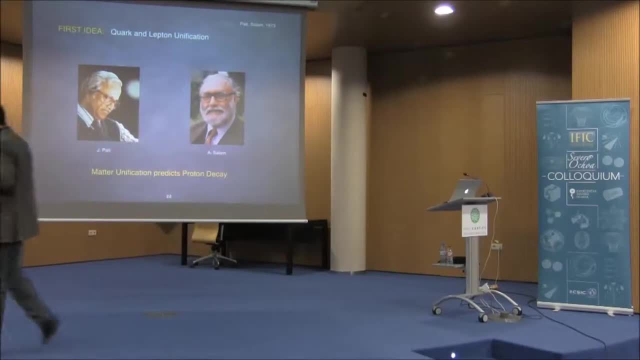 is broken in three units, not in one unit. The problem: when you do that, you put quartz and leptons together in a. we say this in a in a box on a multiplier, this symmetry barren number is broken because you cannot define that. 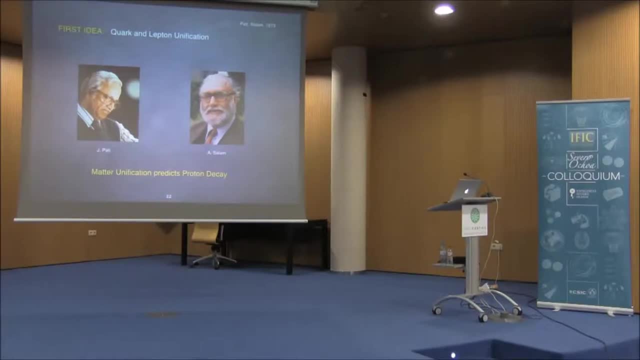 and the scale will unify in matter And therefore you should generically predict proton decay. Later the details are different, Depends which theory you write down, But this is the first idea that actually initiated the idea of unification. Okay, 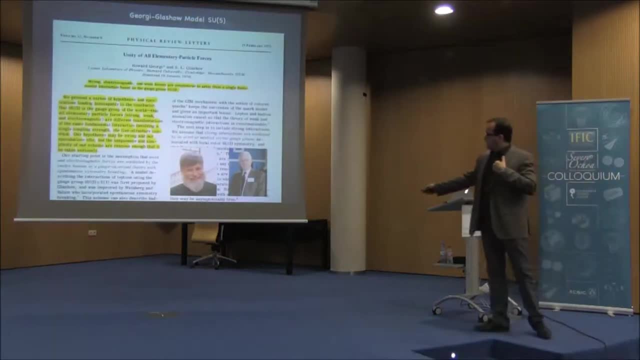 In particle physics And later in 74, Georgi and Glashow, they proposed this amazing idea that the standard model of gauge interaction could be unified in just one gauge group, SO5.. Okay, In the standard model we have SO3,. 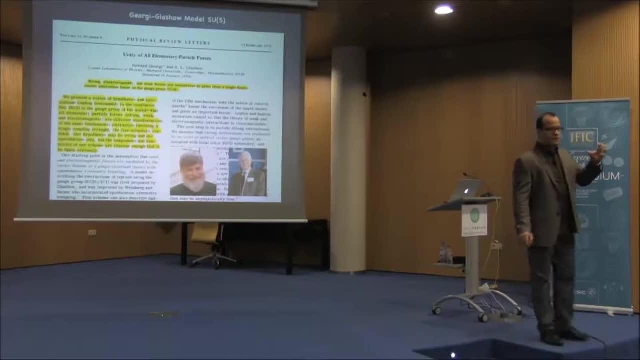 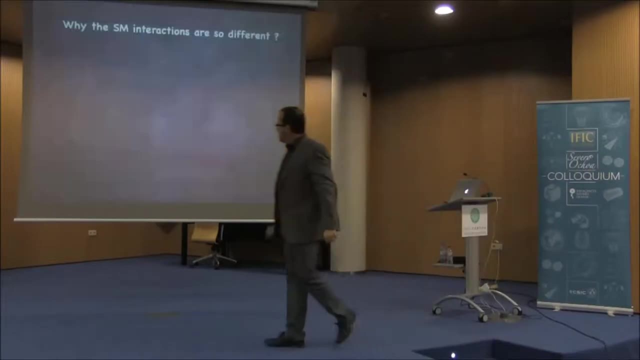 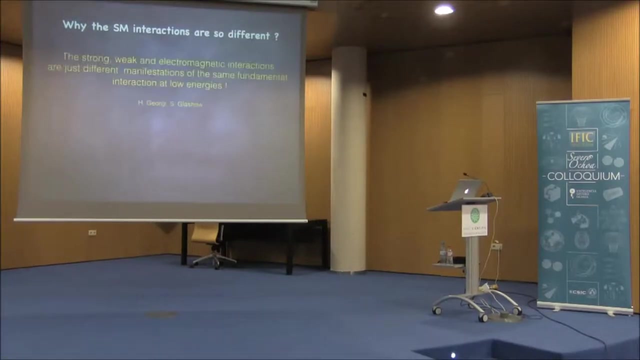 SO2, U1.. Here you have just SO5.. Very simple, Beautiful, Okay, Yes, Simple. And then they have the answer to this question Why the standard model interactions are so different. The answer is very simple. 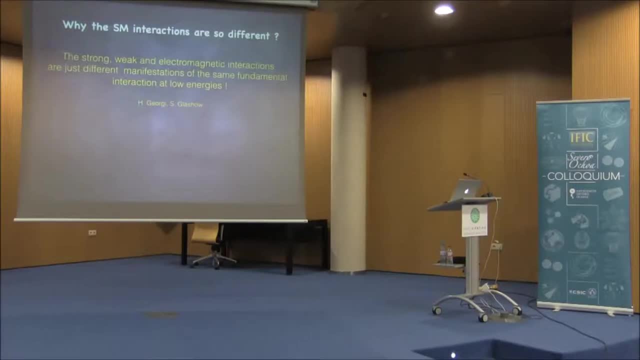 They say, don't worry, The strong, the weak and the electromagnetic interactions are just different manifestations of the same fundamental interaction, of the low energy. Then in a low energy you see that they have different values. Or the mother feels the different interactions. 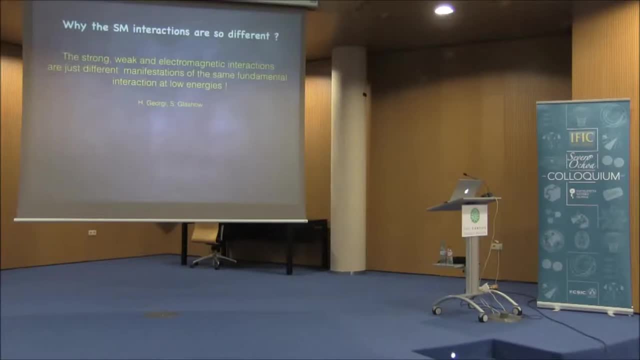 in a different way, But if you go to high energy, they will feel just one force. Okay, They will feel just one force. It's impossible to go to super high energy Because when you do, you study this more in detail. 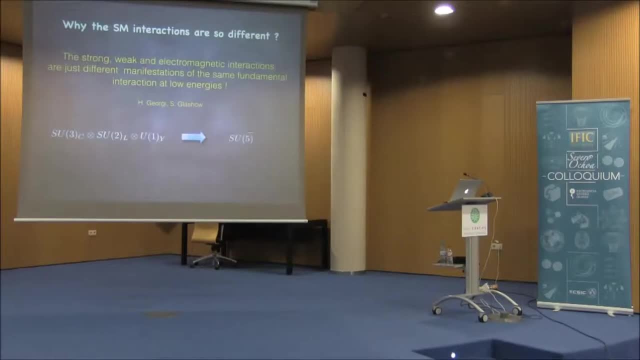 you say very beautifully, I can unify this in just one group. This is very, very simple. Okay, And we know that the energy scale where we can do well with the standard model is below or around 100 Gb. But I told you, 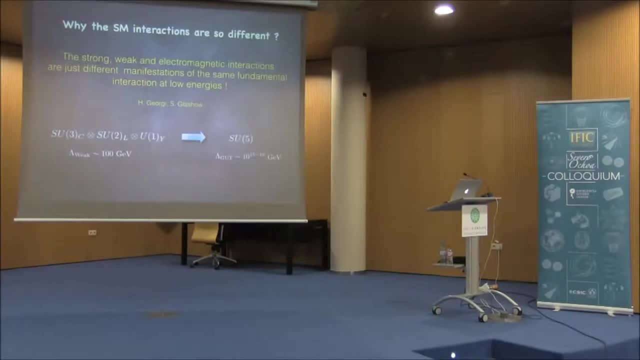 that if, generically, you fall apart as a land, as I will show you, you will get proton decay, and this symmetry cannot be realized at this energy scale. It has to be realized at the super, super high scale. Okay, Which is very depressing. 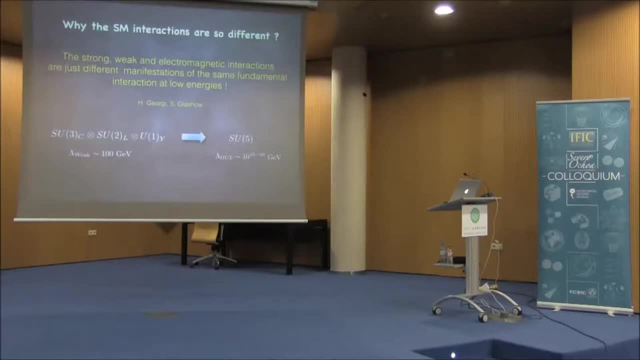 Okay, Because the idea is very, very beautiful. It's hard to imagine. I recommend any student to read this paper. It's a bit interesting because they say that they are totally convinced this is the symmetry of the universe. But you know, the point is that 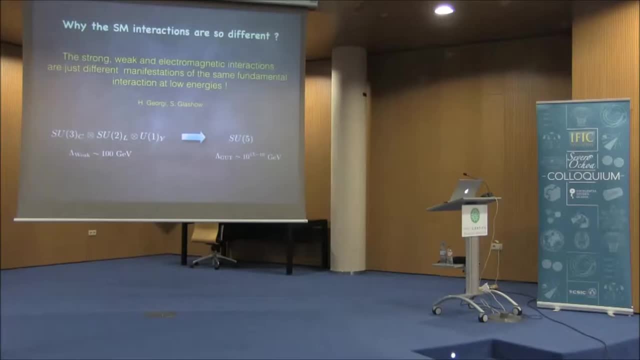 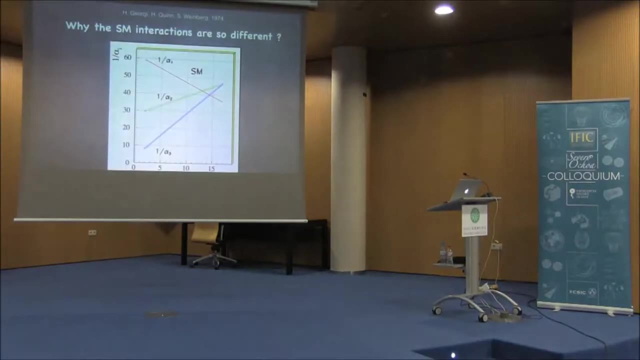 the experimental result tells you that maybe it's true, but you have to realize this is the super high scale. Okay, And then this is just matching the idea, the result of St George, Elling Quinn and Weinberg that they saw very naive. 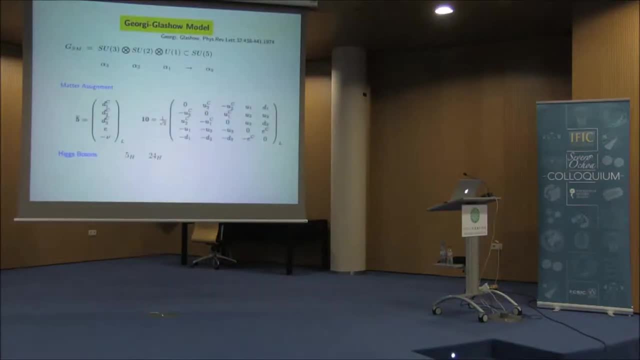 at that time, the unification of the super high scale. Okay, And then, of course I am not allowed to give you details in a colloquium, but at least for you know, to give you interactions in one gauge group. you will have only one gauge coupling. 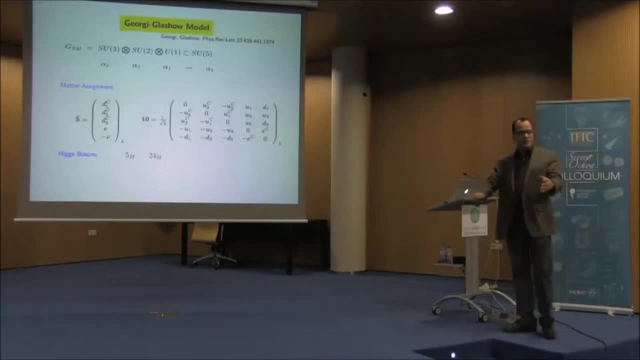 in this case, and the quarks and electrons. they live together in two representations. But the important point is that you put quarks and electrons together and they are at that scale where you have the symmetry. they are no different anymore. Okay, And again the 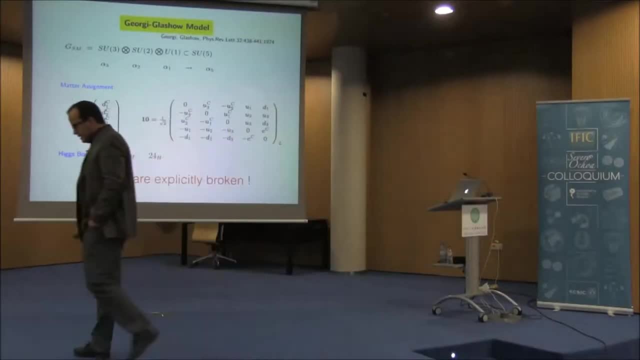 when you do that, because you say it's very beautiful, I like to unify. when you do that, this symmetry is of standard mode because the numbers they are broken specifically because you are forcing the quarks and electrons living together. They have different properties once you put together. 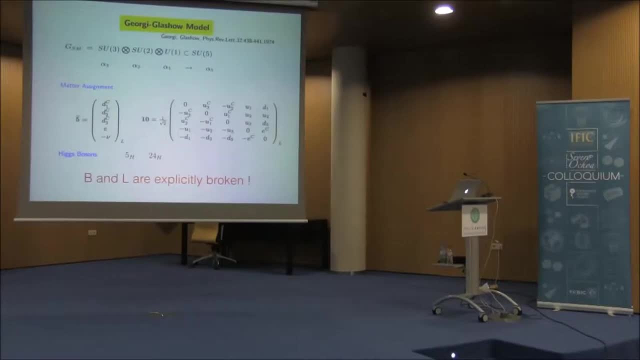 they cannot share the same property, And then this barrier and electron numbers are totally broken. Okay, At the scale where you have the symmetry now, Then this has, as I mentioned, huge implications. There are new fields in the theory. this doesn't. it's not relevant. 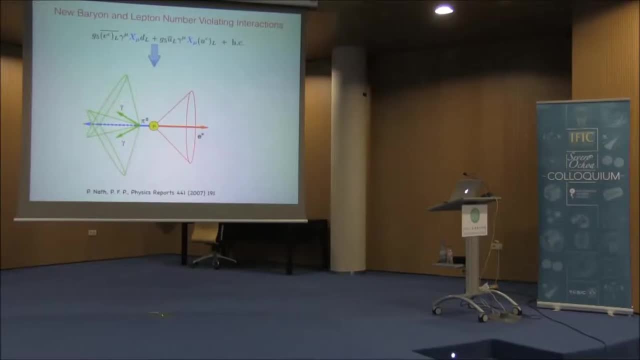 for this discussion just mentioned The decay of the proton, For example. the proton can decay to a positron and a pi zero, which gives you two photons. And then this idea was so impressive- and has still is very, very appealing- that since 74, the experimenters 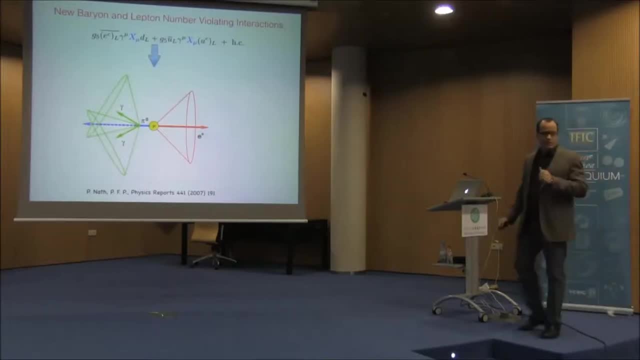 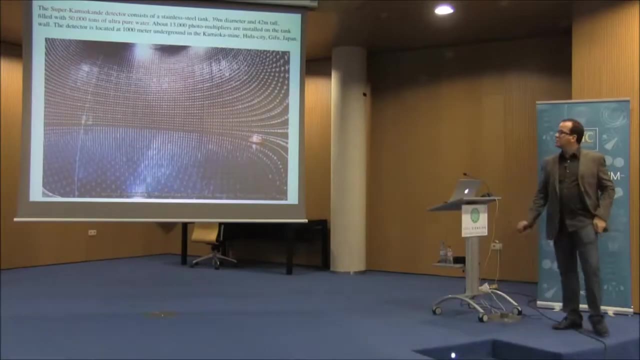 they got crazy and started to build detectors and detectors and detectors. This is one of the detectors. Okay, This is a chemical, chemical detector which is has only 50,000 tons of water. Very small right Has like 30, 13,000. 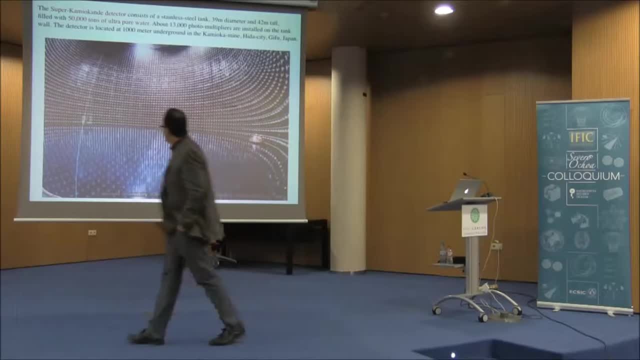 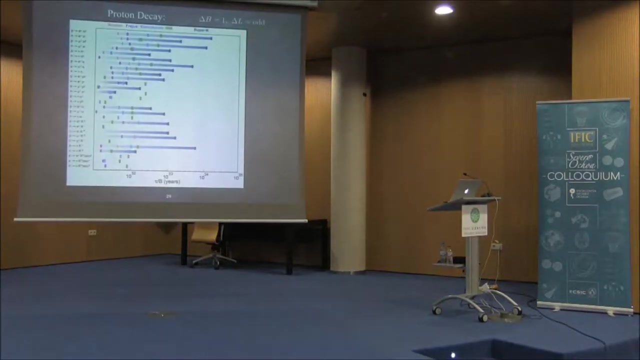 photon multipliers. You see, You can actually swim inside if you want. And what they do? they just wash the proton with water to see if they see a decay from the proton. Okay, And they have been doing this for a long time. 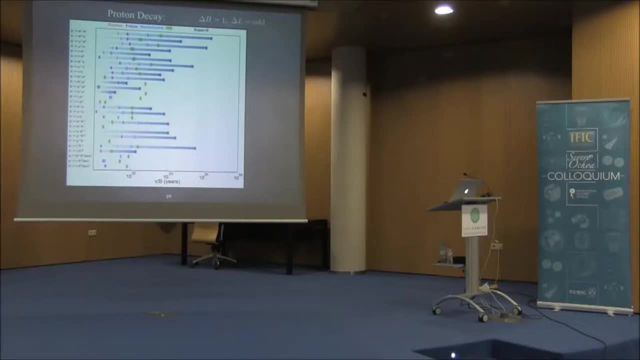 Okay, It has the best bounds that we have in particle physics. This is a list of channels, Huge amount of numbers. There are many, many collaborations, but I will just show you two. Okay, Look, This channel is bound. the lifetime has to be. 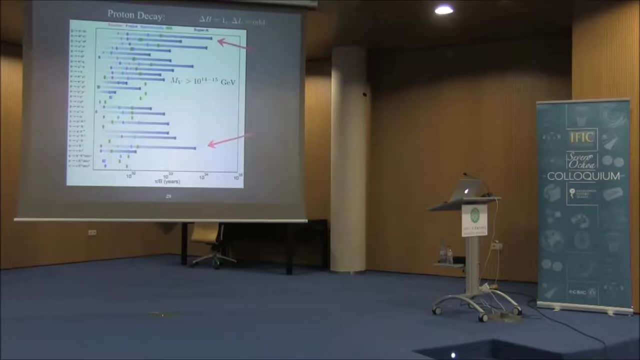 above 10 to the 74 years, This one as well. And when you do take this into account and you compute the proton lifetime in this theory, I tell you that the new gauge fields mediating proton decay or giving this process. they have to be. 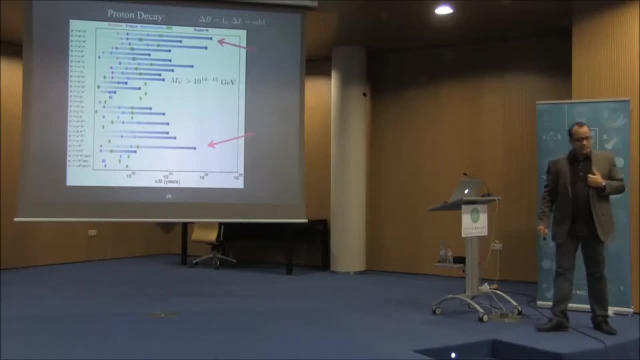 super massive, Okay. And again it's depressing Because you say, okay, beautiful, I can unify SO5.. Great, SO5 gives me a prediction, a new prediction in nature, which is the proton decay. Very beautiful, But I don't see proton decay. 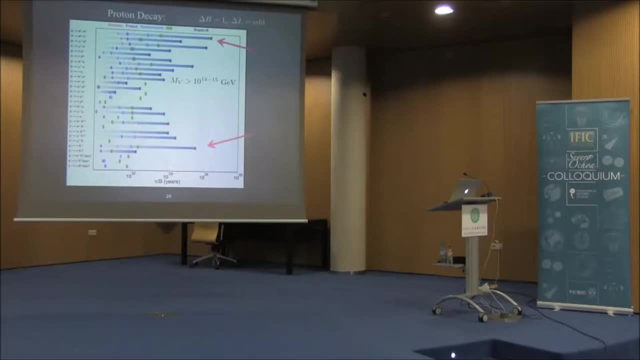 and the theory has to be at a super high scale. Okay, Depressing, Or maybe nature is like that. Okay, And this is what, for a long time, we call this, for more than 40 years: physics at the high scale, Maybe like a dream. 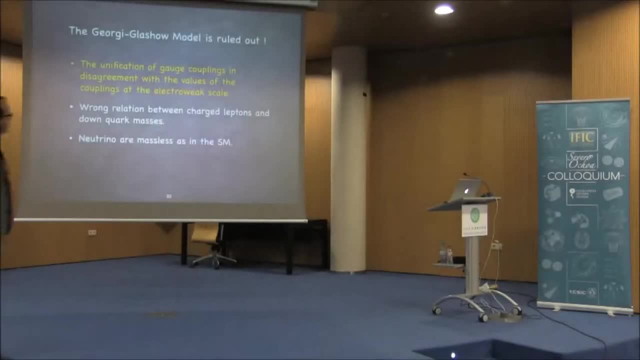 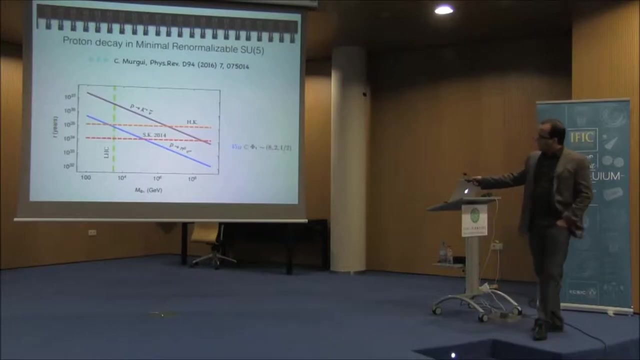 maybe, But somehow many people like that. Okay, This theory doesn't work very well, but you know it's good enough. You can accommodate many things, many of the problems. For example, this is a a a prediction that I have when my Clara dies here. 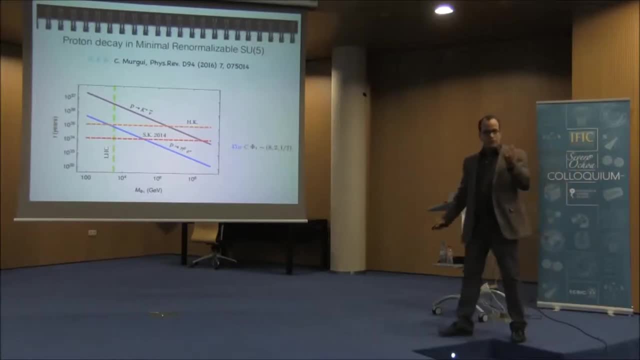 You can actually write a theory that is totally realistic, You can explain, you can have a consistent relation for Fermi muscles and everything, And you can compute the lifetime of the proton, And this is, for example, for the positive. you can actually do a very good. 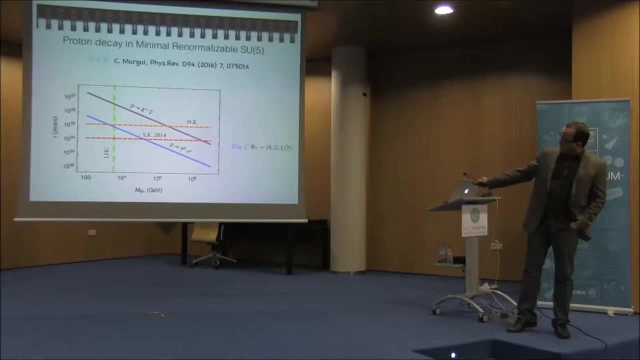 calculation. You can use the super and you can see that. if can, actually this is the projection for which is the new generation beyond super k, you could see maybe a way to see if this theory is true. you could imagine that the upper, you could see a signal. 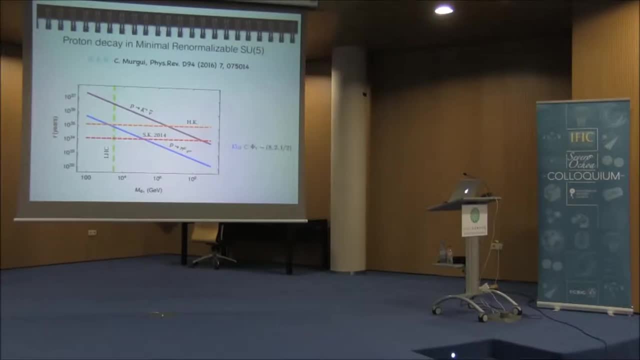 Okay, But again, even if you see proton decay, okay, you will make a celebration in Japan. you will drink maybe a lot of sake, I don't know, but this is a new phenomenon in nature- the proton will decay. this is pretty amazing, Okay. However, you cannot. 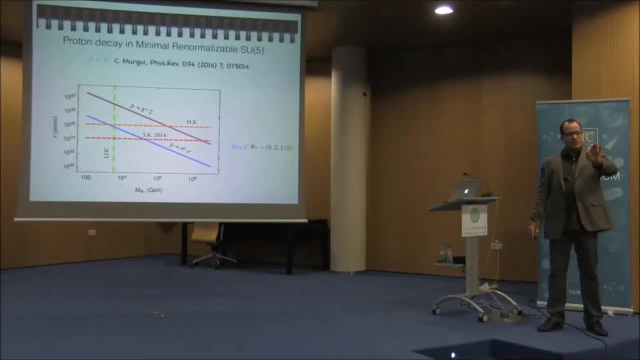 go beyond that. you cannot say this prediction corresponds to this very well defined theory because in reality when you check that is super high, super difficult to make a conclusion. you can say you can maybe rule out a theory because we cannot produce the fields that are mediating. 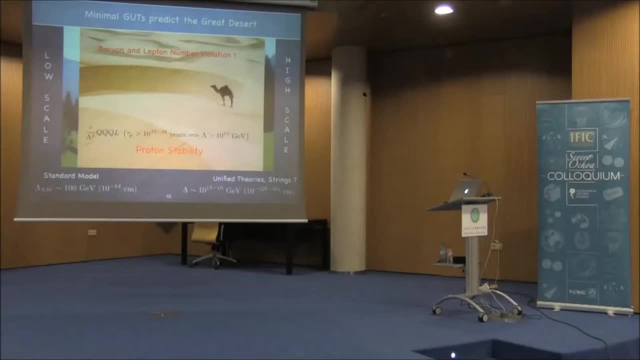 proton decay in a collider. we never can really test a grand unified theory. Okay, And then you live in a very funny scenario regarding unification. you know, we know that we have the standard model here, very light lower scale. no, I told you proton stability. 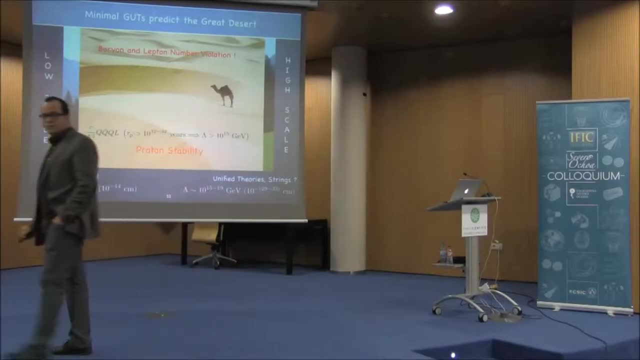 generically will tell you that your unified theory doesn't matter how pretty it is, how, when it doesn't matter. you had a coffee with tea when you wrote. the theory has to live on the super high scale, Okay, And the large upper collider can, maybe. 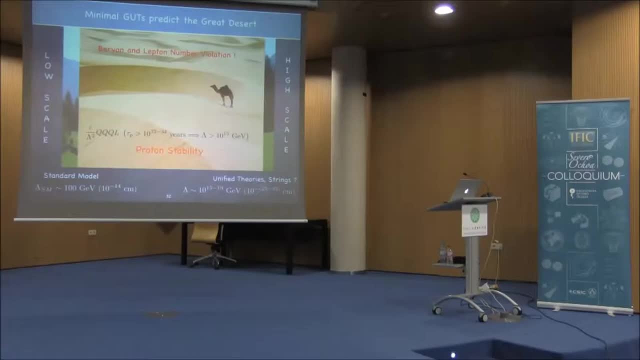 prove. this region here at the TV scale is called the Great Desert Hypothesis. So you have two physical scales that are far each other, really far, and the only thing that tells you that this has to be like that is just the fact that the proton 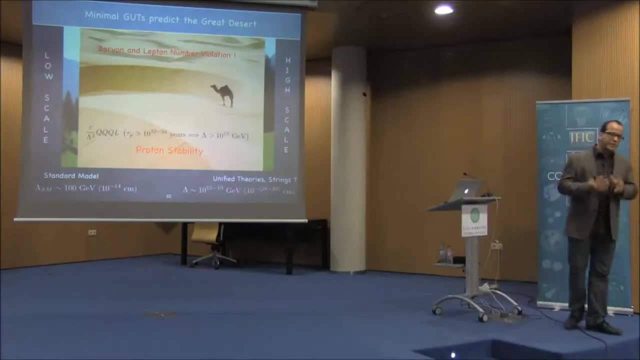 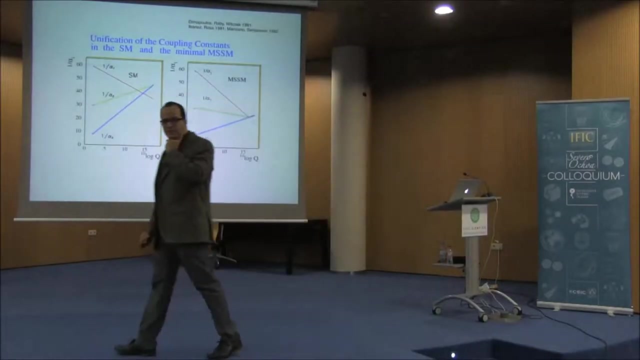 doesn't lie to decay. Okay, Just doesn't lie to decay. The bounds are pretty amazing, The best bounds in high energy physics. Okay, This is the story about the ideas of theory and proton decay. But you know, we get really, we like 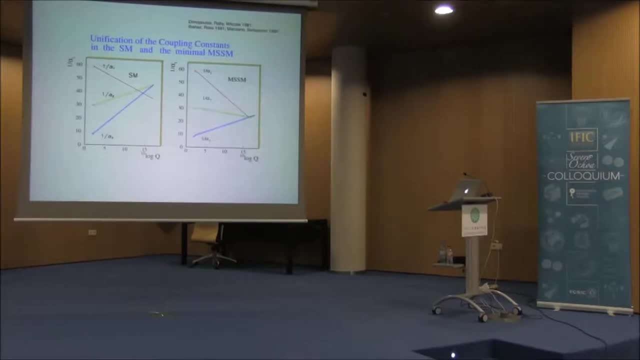 to play even more than that. And there are more ideas like supersymmetry. Okay, Supersymmetry that people like for many reasons is a very beautiful thing, because they didn't really know even the values of the gauge couplings. Today we know. 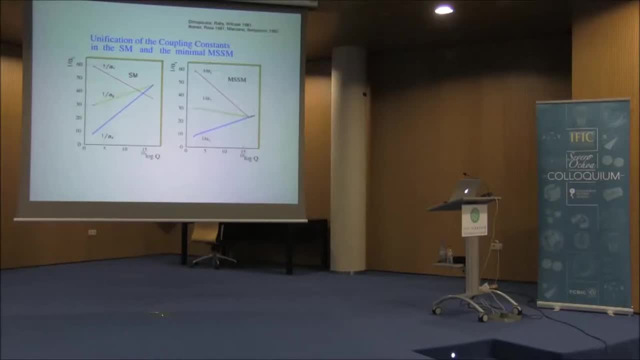 this doesn't really work. Doesn't really work. And when you use supersymmetry at the lowest scale, you find something very interesting: that you actually can meet these couplings at the super high scale, which is super high scale. And, of course, once you know, 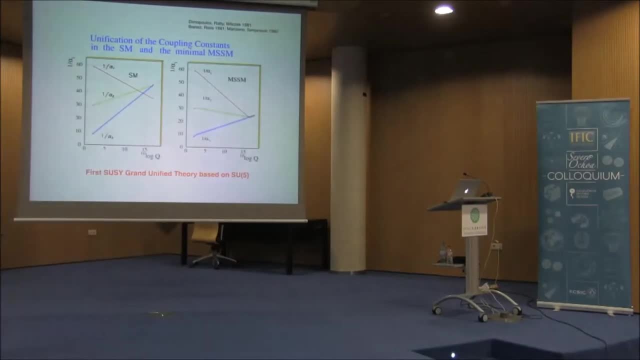 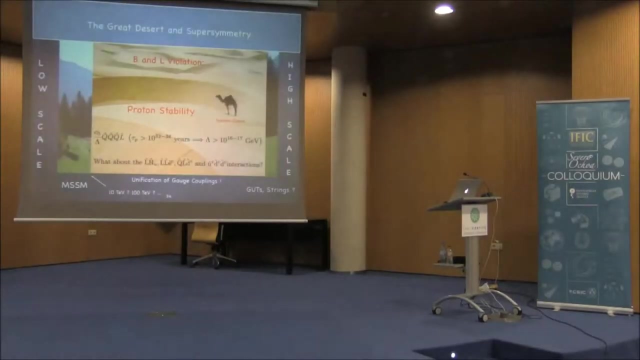 supersymmetry theory, and you already knew SO5. the same father of SO5 wrote the supersymmetric theory. Okay, Just one step forward. Okay, Just putting supersymmetry in the game to help more to achieve unification, in agreement with experiments, in that case. 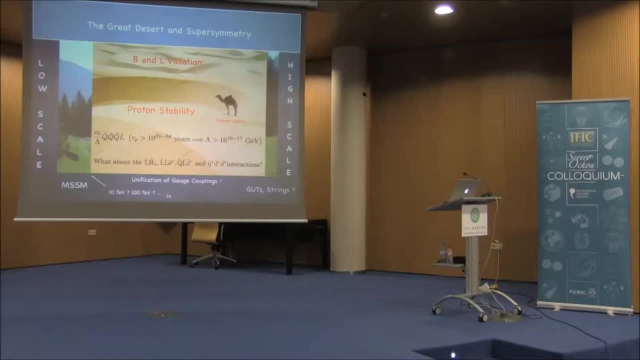 the situation is a bit different, because maybe you can find the supersymmetry extension of the standard mode at so low energy scale. we have no idea. This is just one speculation, just one more idea in the market, But it's interesting, it's a very 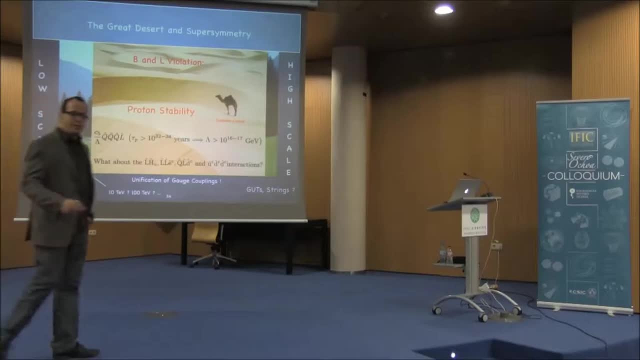 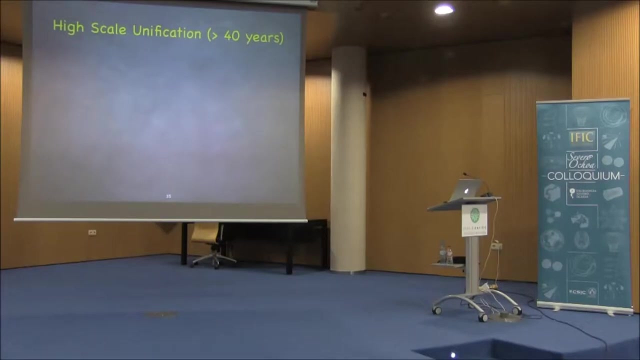 appealing idea because there are even more problems when the proton likes to decay faster and it's actually very hard to accommodate the experimental bounds. Okay, But it's maybe appealing. it's a good idea that maybe, if LHC can discover supersymmetry, you can 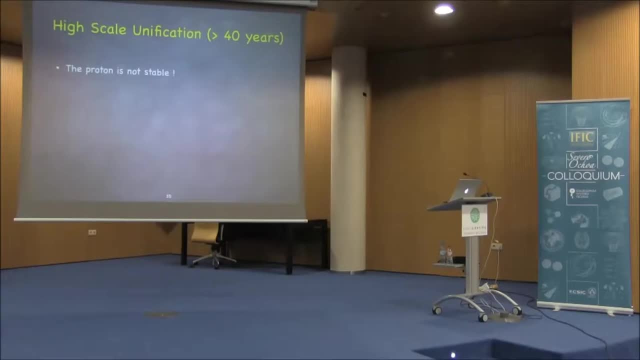 do it Okay, And you have. for more than 40 years. we had this beautiful idea of grand unified theory where you have a new prediction in nature that say the proton is non-stable. You don't have to worry about that because it's. 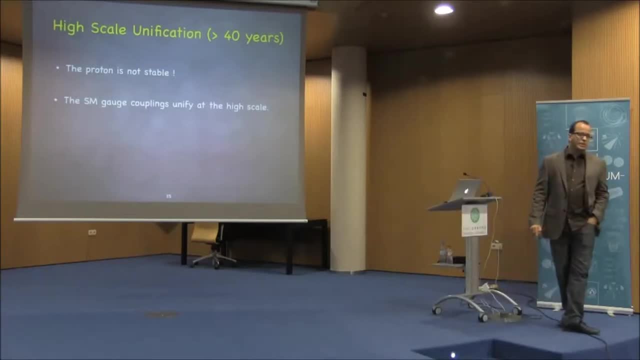 a high scale, which, again, is maybe interesting, but we never will be able to test this in any real experiment. And you can write beautiful theory based on SO5, SO10.. If you like group theory, just play games and build more and more interesting theory. 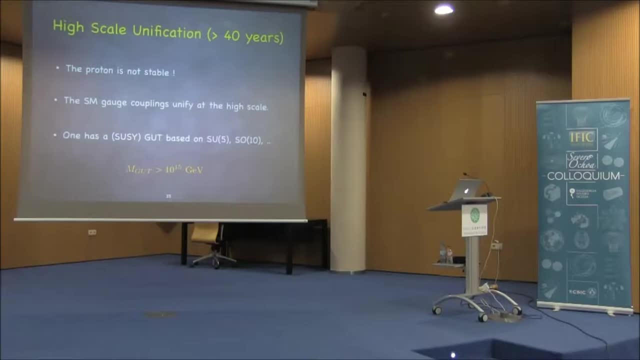 But again, this is super high scale. Okay, Very pretty. Again, if you go to string theory or anything like that, they are talking about playing scale. Okay, That is again very pretty, but we never will know about this. Okay, We never can build. 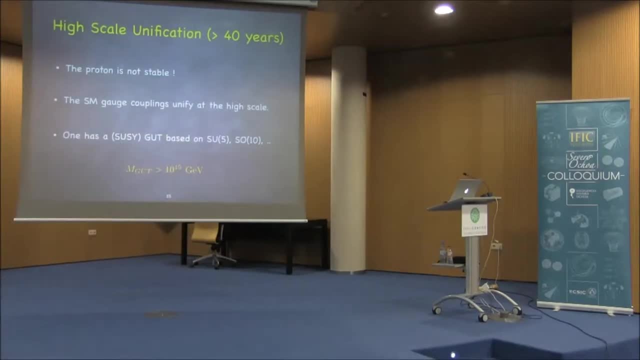 any experiment to test this. Okay, Even if you want to do this experiment, you can do this. Okay, Now let's assume that maybe this story is not true. Okay, It's so beautiful that it will be very interesting to see what happens. 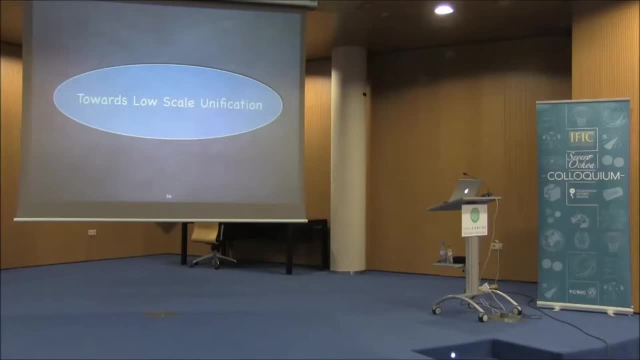 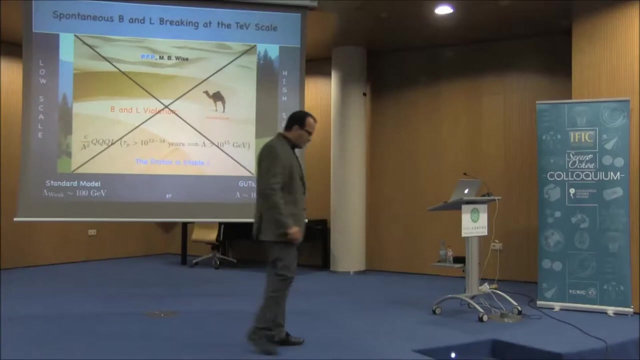 in the future. Okay, So we have to think about super high scale, because I can live 100 years in my lifetime and never will die. But of course the proton has to be stable, because the proton is the guy that drives you crazy in this. 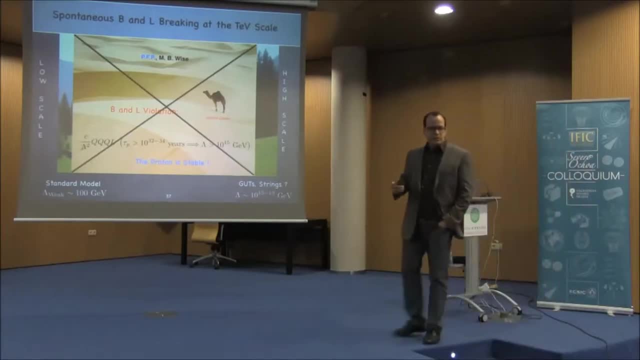 story. Okay, You can do all the mathematics that you want, a very beautiful group theory, but the proton doesn't like to decay. It's just a simple question: Can you write a theory where the proton is stable at any level of perturbation? 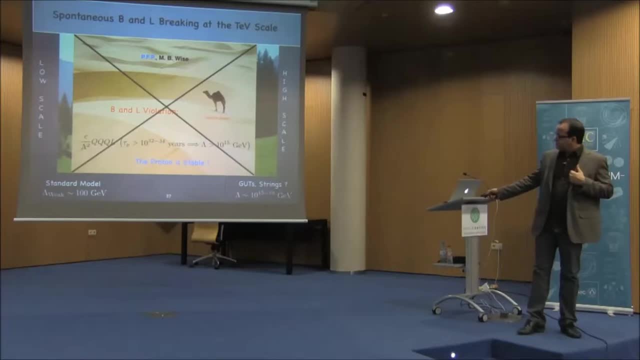 theory. If this is true, maybe this higher scale, you don't have to have unification of the super high scale. Maybe you can unify this. This is the key point, Okay, And this idea is actually related to something different In the 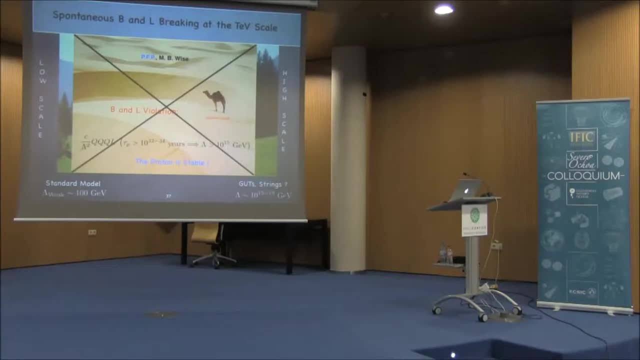 standard model. we understand mass generation is doing spontaneous symmetry breaking. Here I told you that unifying theory: the number is broken by the number of particles in the mass of the proton, And the number of particles in the mass of the proton is the. 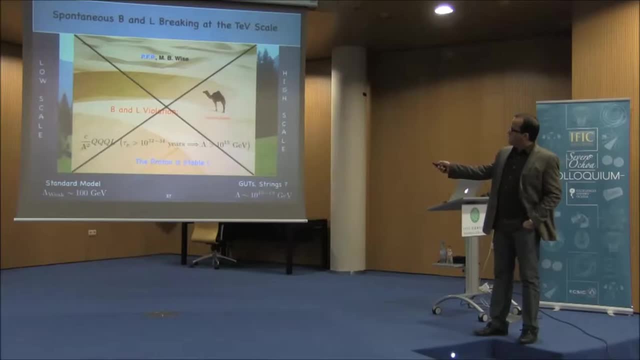 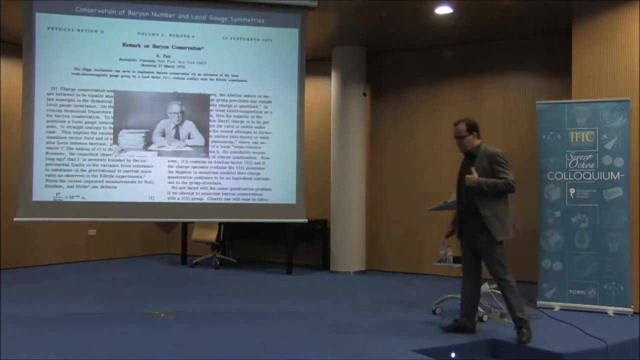 number of particles in the mass of the proton, And this is a very interesting idea, And this idea was hidden in a paper that has like 20 citations. You know, the has like 5,000 or I don't know how many thousands. 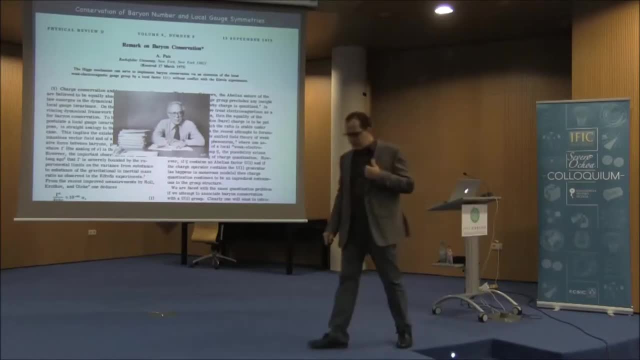 of citations. This is a very interesting thing, And he just wrote a very short paper that says: oh, maybe you know, a number is not a global symmetry, it's a local symmetry, And he just was happy with it And he 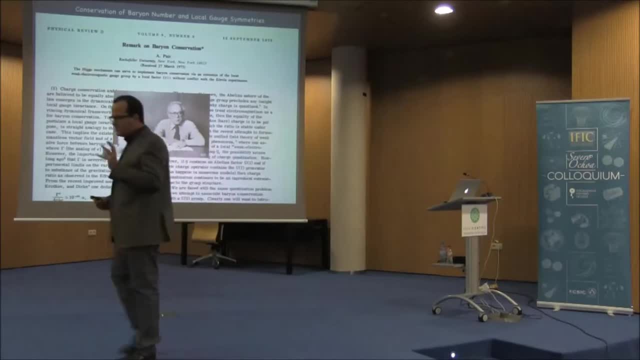 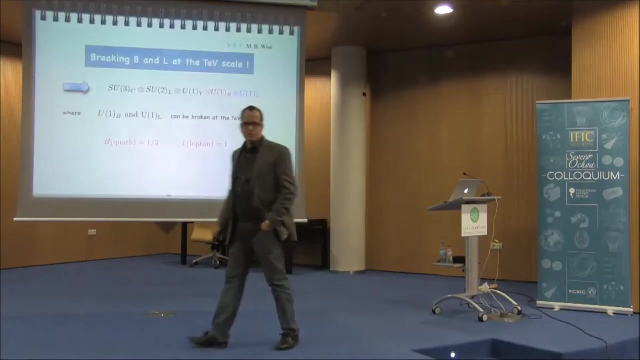 wrote a very interesting paper that he wrote in the paper And he wrote a very interesting paper that he wrote in the paper. And he wrote a very interesting paper. You will find, you will be surprised. there are only a few papers in the. 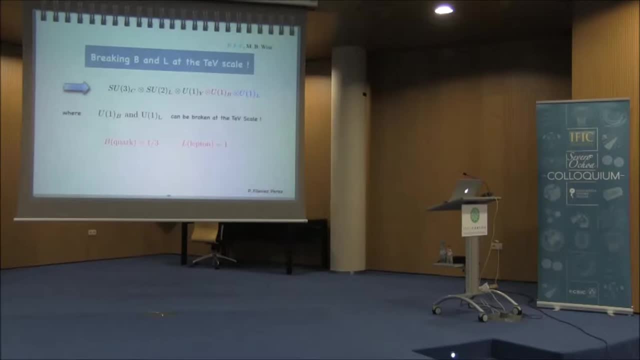 market. Everybody knows this. Okay, In the field of high energy physics. Okay, Let me explain you how you could maybe do that. Very simple. Let me explain to you how you can do this, So you can do this You. 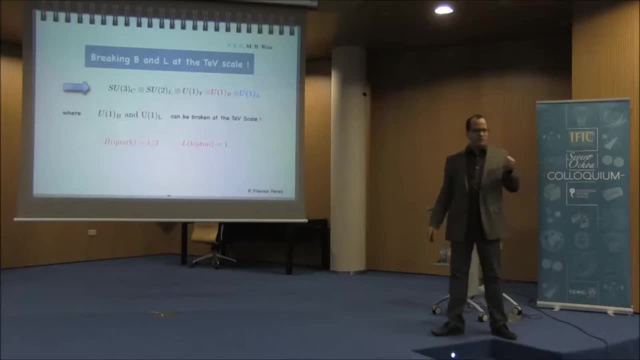 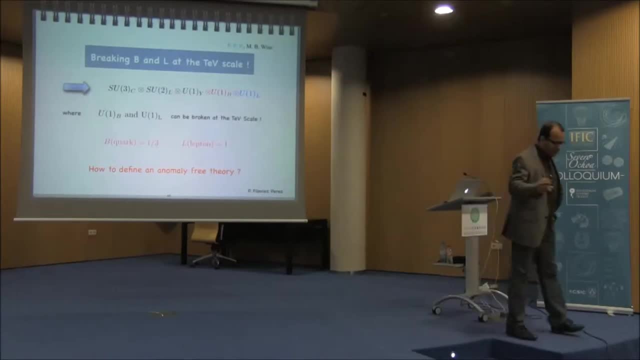 can do this. It is very. If you want to study the spontaneous breaking of symmetry, you have to make sure that this symmetry is good also at the quantum level before you break spontaneously, Because if it is broken at the quantum level you have no idea what you are doing. okay, 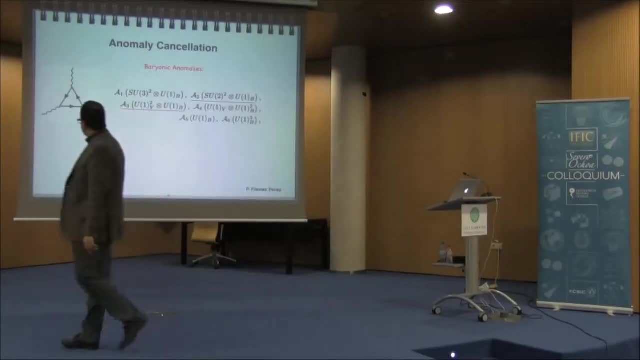 This is something that is called an anomaly. You have this funny graph: three gauge bosons associated to a varying number and inside you have fermions. inside, In this case, only the quarks, because the quarks are the only ones that they have a. 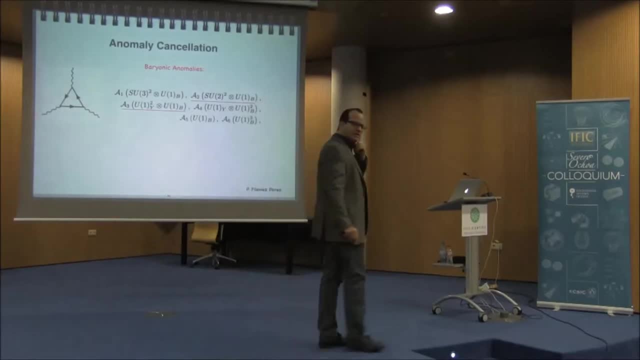 varying number and you have to check all this graph and make sure that somehow they are zero. If not, it doesn't make sense to understand the spontaneous symmetry. breaking The standard model is so impressive that when you write all the multiple quarks and lettuces, 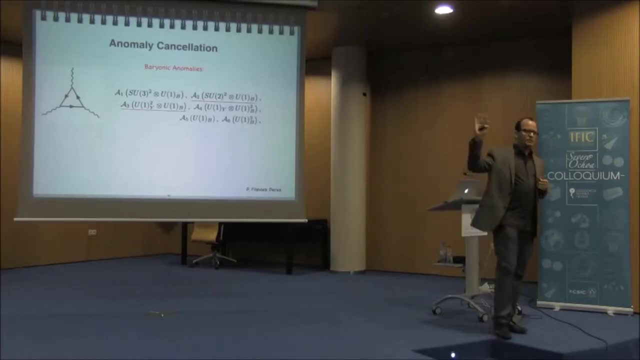 and use all the quantum numbers. all these graphs are zero automatically. This is so much. this is what is called the standard model of particle physics. you know Well, if you check that, you know you realize that the situation is not really so bad. 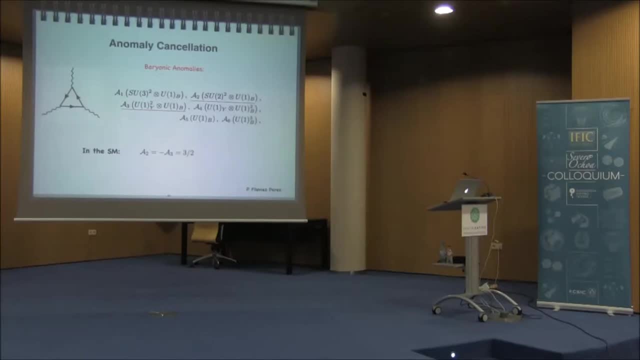 You realize that there are only two anomalies. okay, I don't want to be technical, but basically there are only two types of graphs that are not zero, And you say, oh, that doesn't look so hard. okay, You do this before lunch. 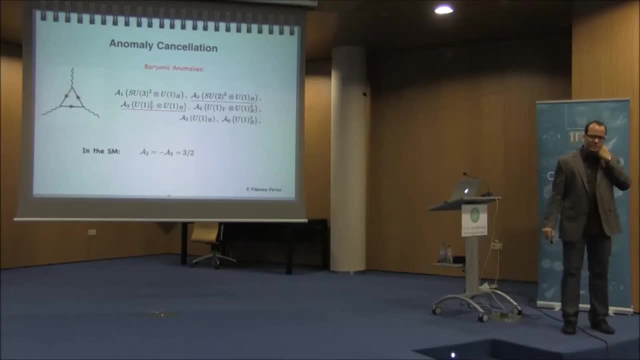 Go for lunch, Come back, The lunch is good, You keep going right, The food here is good, Then you're fine. And then you check and you say: okay, maybe I can do a job, I can write a theory for varying number and this symmetry is anomaly free. 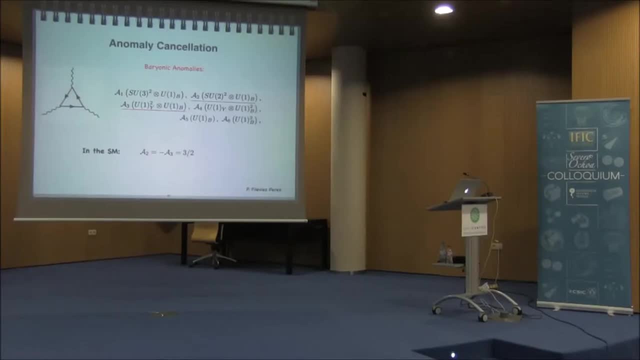 And then I can understand the spontaneous breaking. I break and see what happens. I cannot give you the whole details but, believe me, we try everything possible, everything human being That we try, And the LHC did kill two possibilities I mentioned. you cannot have families that are similar to families that we have in the 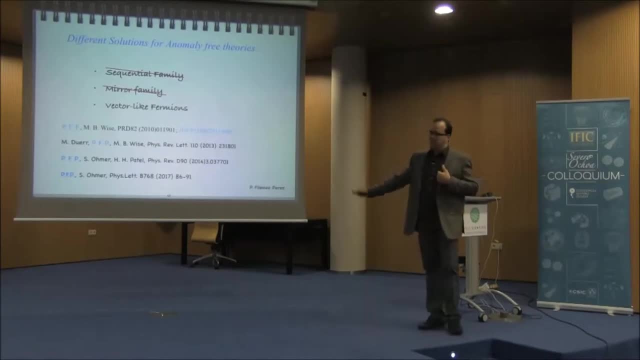 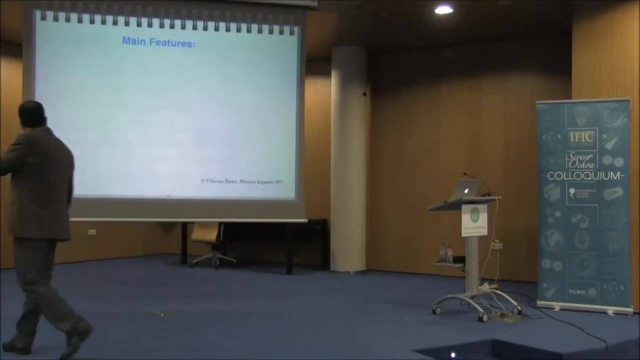 standard model, You can have something that is called virtual life fermions. It's something that doesn't care too much about chirality, you know. And then, before I give you details, let me give you the main conclusions of this SSI. 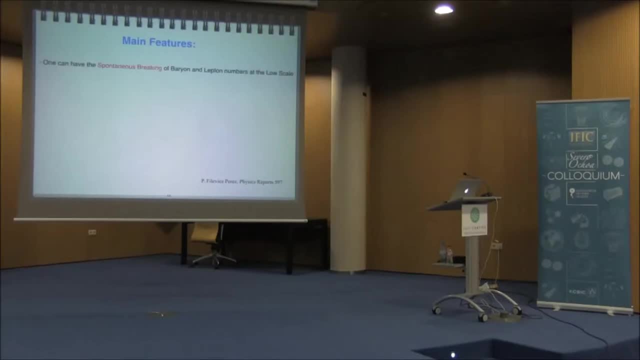 which is that you actually can show, that you can actually have. you can have the spontaneous breaking of the symmetry at the lowest scale. You actually can do that in agreement with cosmology and any particle physics experiment. You predict a new gauge boson. 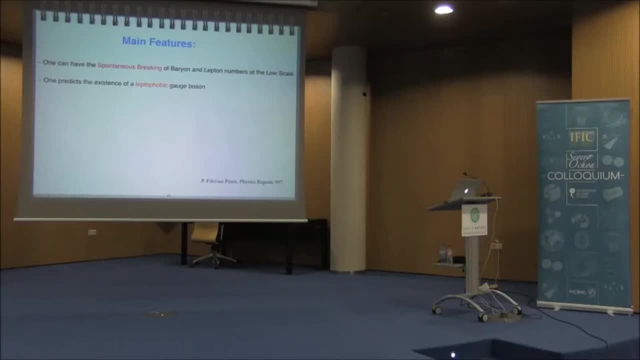 It's like the photon but it's massive, or couples only to quarks, which is has very interesting properties. You could you produce a. you have a new, like a Higgs boson with funny property we call baryony. 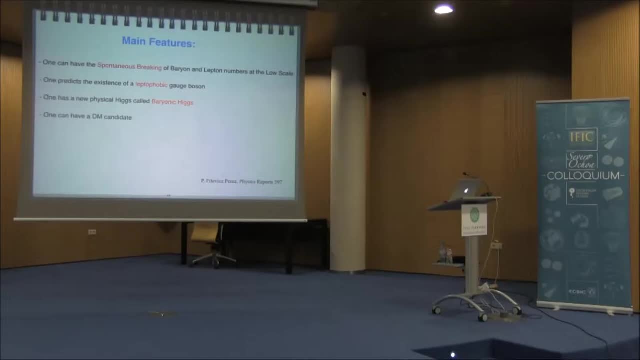 Because it has to do with the spontaneous breaking of baryon number. You find a dark matter candidate here and we were looking. we were not looking for any dark matter candidate, because I never told you anything about dark matter here, right? I told you just a proton is, a is a troublemaker and you want to understand the stability of? 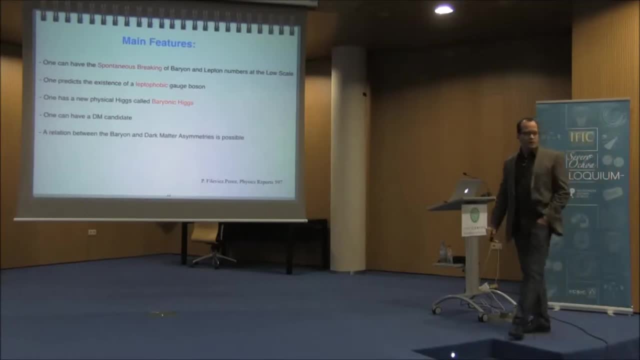 the proton, You can show that you can actually explain even the variance in the universe. and, as I told you, the key point is that if the proton is stable, You can start dreaming about unification at the lowest, at the lowest scale. okay, 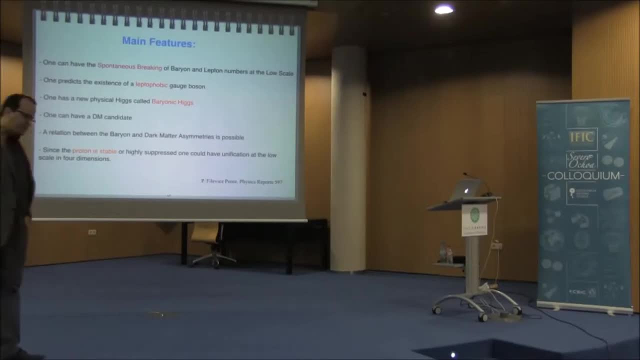 Because, again, I told you all this idea of Georgian glaciers are very beautiful, but they can be only realized at the super high scale because the proton is not stable. But here, if the proton is stable, again you start dreaming about changing the game. okay, 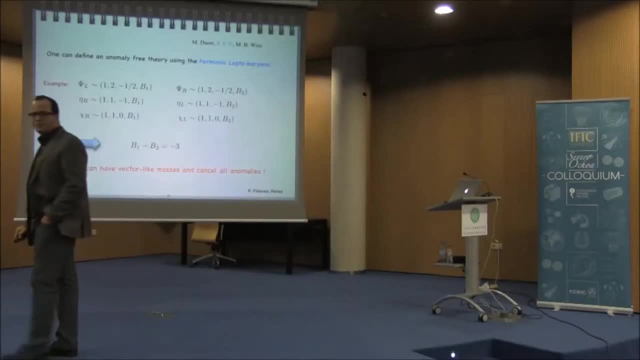 Okay, this is like the simplest, simplest, simplest model that maybe for some of you is really complicated, But not really complicated. Okay, They are like only three fields: fermionic fields and the particle life partner of these guys, But it's not even relevant for this discussion. don't even look at this. 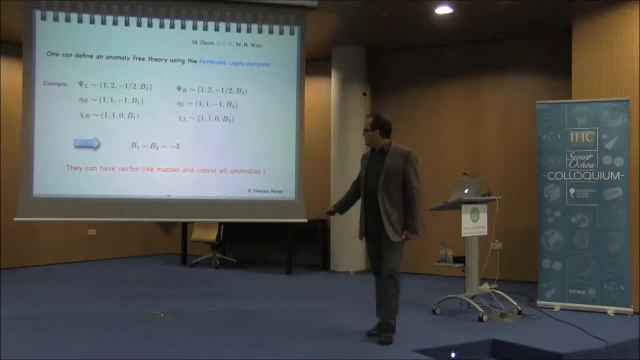 The only thing that I want you to look is that these are the barrier number of these fields And when I check this anomaly, this graph with three gauge bosons and all the fermions inside the loop, I want to cancel that and make the theory. anomaly free means that the 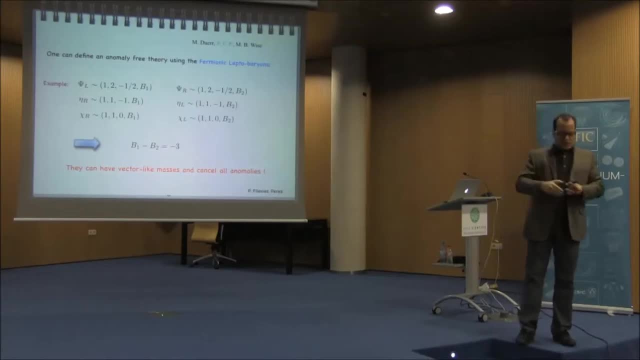 quantum level is not broken And I want to understand the stability, I want to understand the spontaneous breaking And I find a funny conclusion is that the difference of this barrier number is minus three. And this is interesting because, I told you, in the standard model of particle physics, 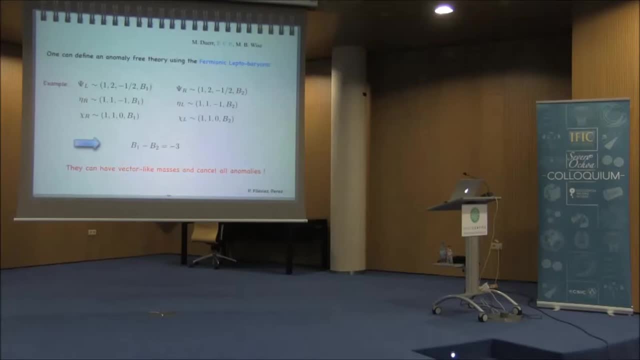 barrier number is broken in three units. The proton is stable because the proton can decay only if you break barrier number in one unit. You can think about that. the proton can decay to a photon and a positron. The photon doesn't have barrier number. the positron doesn't have barrier number. the 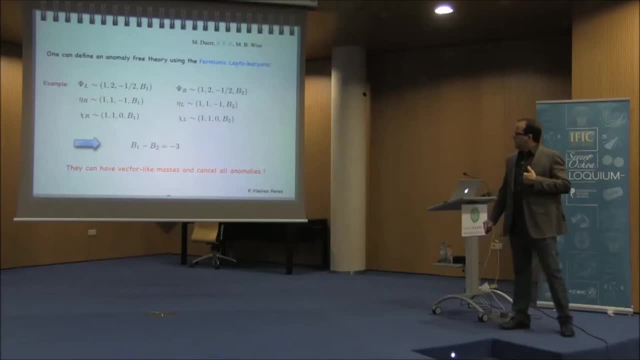 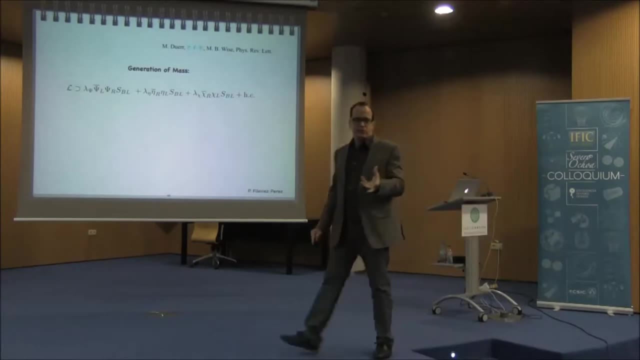 proton has barrier number one. Okay, Then of course these new fields. you have to give mass to these fields because they have, for example, electric charge And we have experimental bound from collider physics. we cannot have a live field in electric. 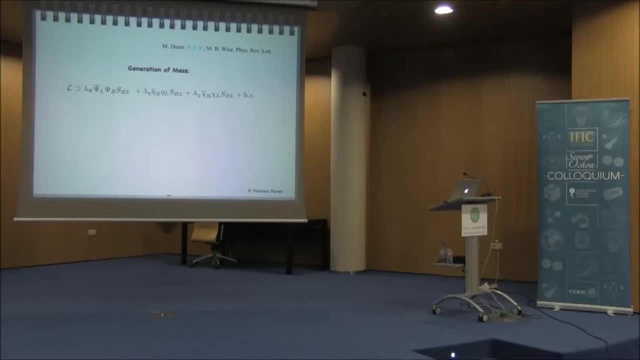 charge. Okay, Then if they have electric charge they have to get mass. But they cannot get mass from the standard model Higgs because you destroyed the standard model Higgs property. Then you have to introduce a new Higgs to break the symmetry and give mass to the new. 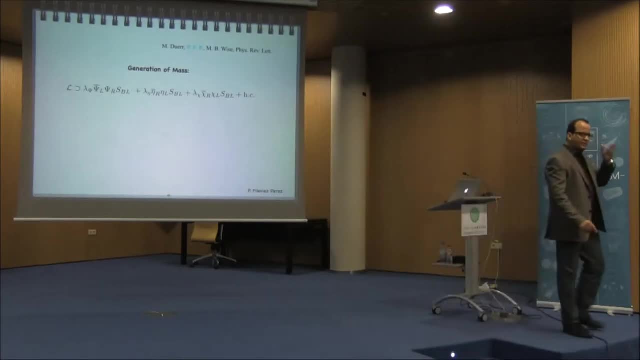 fermions And you will tell: okay, this is just a game, you just put the Higgs and you are done. Well, it's actually not like that. The funny thing is that you find that this Higgs is forced to have a barrier number, which. 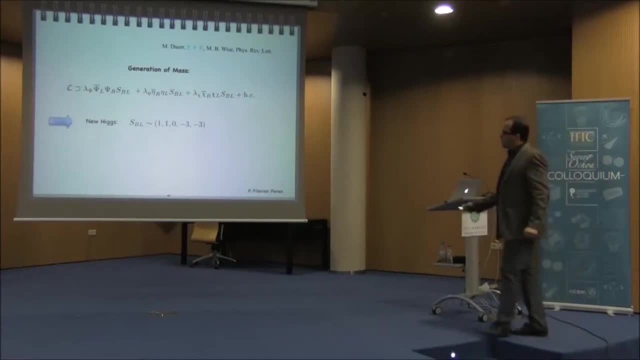 is minus three. Okay, If you want to really generate masses, Because the difference of the barrier number of these fermions are constrained by this cancellation of anomalies, Then if you have that, Okay. This means that you can break this symmetry, but only in three units. 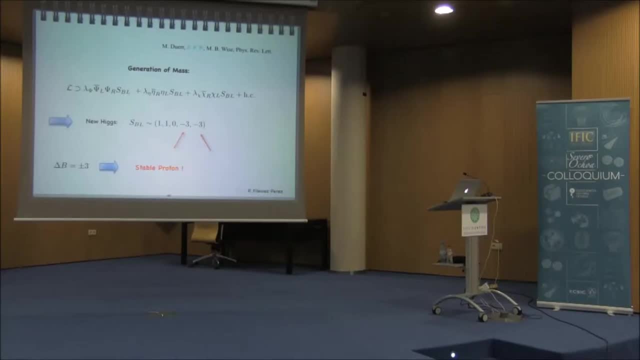 This means that the proton is totally stable. there's no way to generate proton decay here, even if you have the spontaneous breaking of barrier number. And I told you you don't need to assume this desert because proton is stable Now you don't have to worry about somebody that is far away from you. 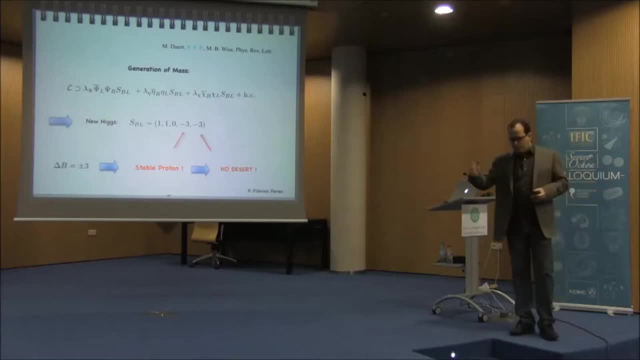 You can start thinking that this can happen on any scale Because the proton doesn't decay. In theory, And I have to say this is a very simple question- Can I write a theory to explain the stability of the proton, assuming that it doesn't decay? 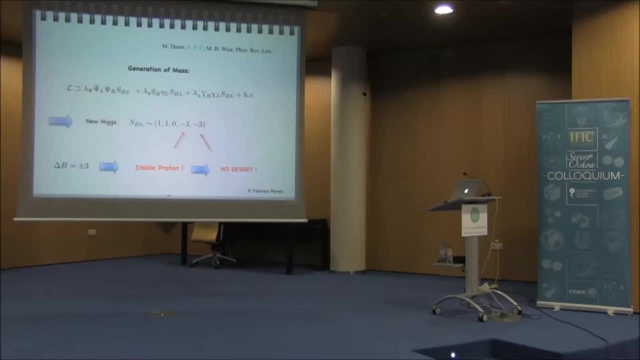 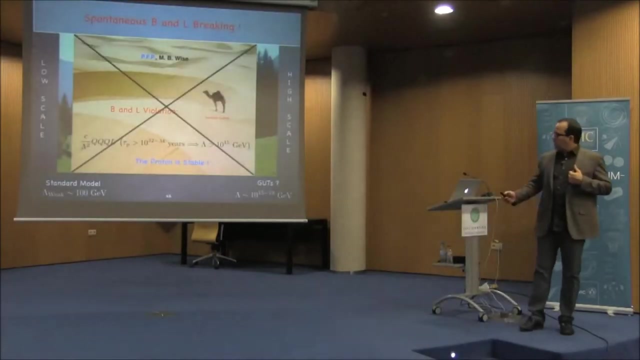 Well, this is the way. Using the recipe of the standard model, Using spontaneous symmetry, breaking Of course, you can assume it doesn't decay. This doesn't make sense. I have to explain things, Okay, And this is why I told you. 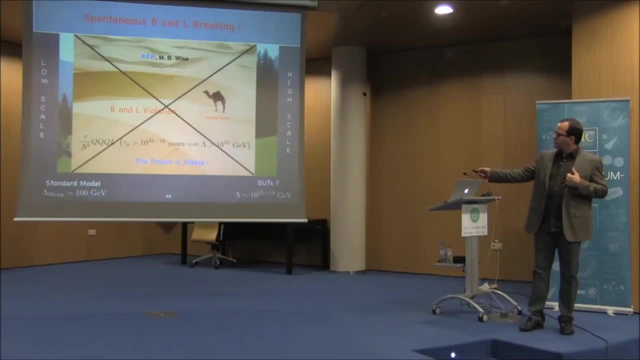 I told you, if you have a spontaneous breaking of a number, the template theory tells you that the proton is stable and therefore this breaking can happen at any scale. it doesn't need to be at the super high scale. okay, And then you don't need to have these two. 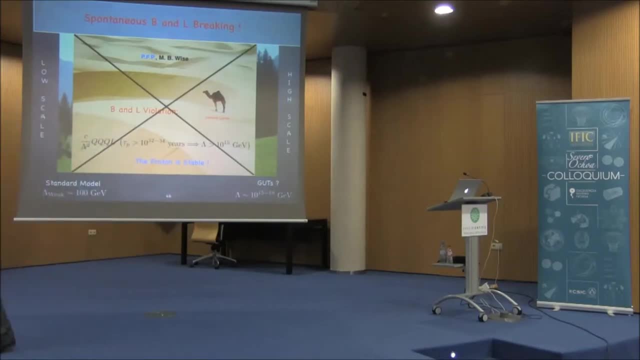 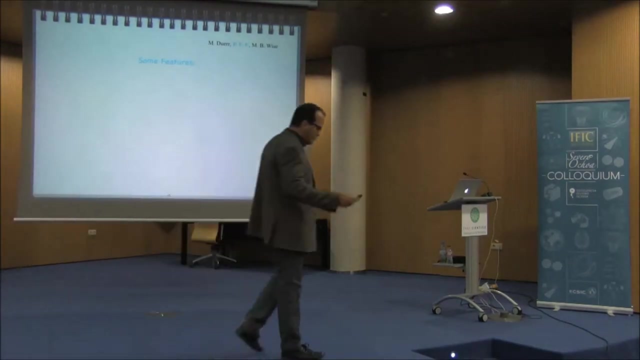 scales far away And maybe, if this happens at the low scale here you can test at the large Hadron Collider, for example. Okay, Maybe Now you keep going And I told you just do this and say, oh great, the proton is stable in the theory. is there something more? 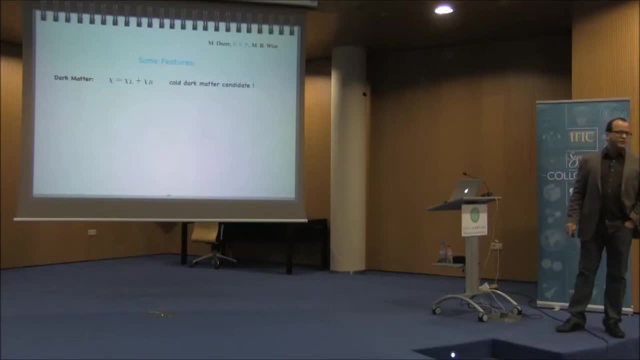 Yeah, You find that there is a dark matter. candidate for free. You didn't look here for any dark matter. You find the gauge boson associated to this spontaneous breaking and all the things. I don't want to bother you, but the funny thing is. 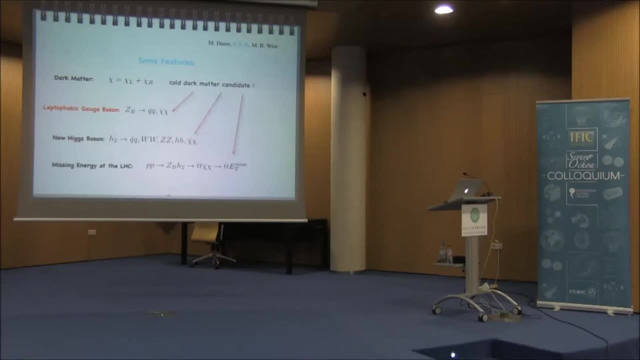 you find the gauge boson associated to this spontaneous breaking and all the things. I don't want to bother you, but the funny thing is. But here you find that all the signals that you could imagine a collider has to do with barrier number and that matter. 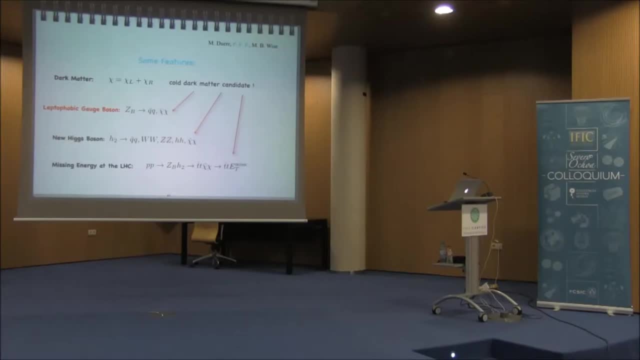 You get that matter everywhere. And this is interesting because maybe you can look for two things: for the spontaneous breaking and the barrier number. And now let me tell you- you can ask me, okay, the Large Hadron Collider started to look for that. 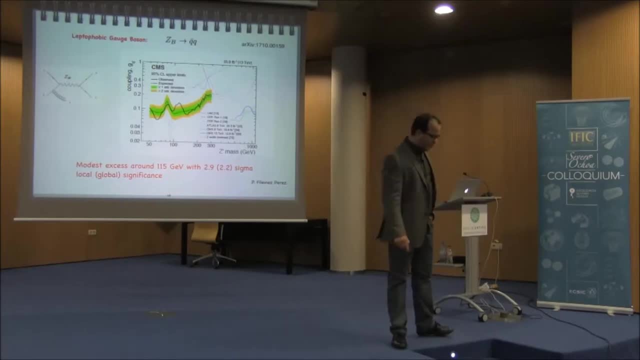 Actually, yes, for a while They didn't have maybe the same motivation. they didn't care about proton decay or anything like that. But yeah, you can see the Large Hadron Collider put now much better bounds on the coupling of this gauge. boson that has information how the barrier number was broken. 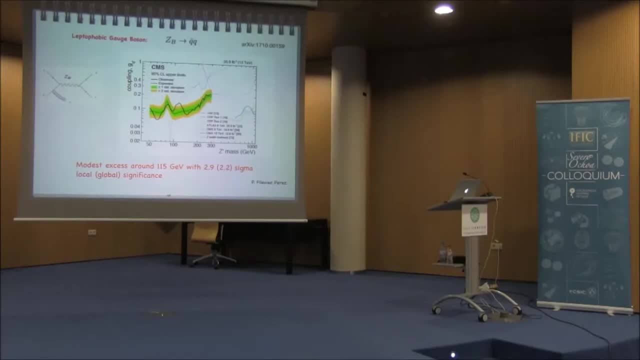 And this is the mass of the gauge boson. But the interesting thing here is that the bounds they have- you know they have a lot to do- They are not so strong. This means that this is, even if this is happening at the lowest scale, this doesn't need to. 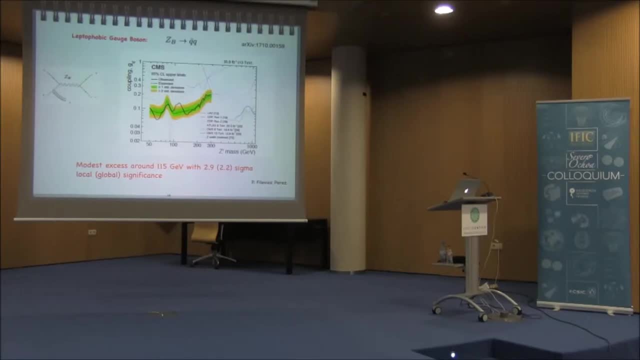 be like a marginal theory where you have to kill couplings and do gymnastics to satisfy experimental bounds. No, you can actually satisfy all the bounds very easily, okay, And the funny thing is that they see even a very small excess there. but this is a joke. 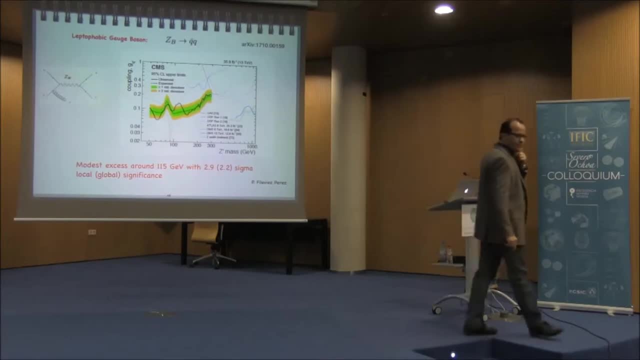 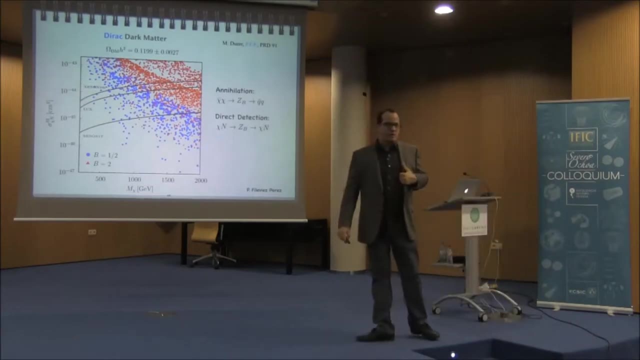 okay, Don't write a paper about that, please. Sorry, People write paper for less, but don't do this, please. Then what about that matter? You know, I guess there are people here working on that matter, also looking for that matter. 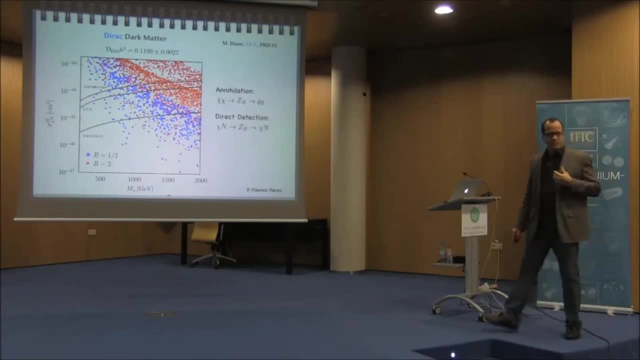 experiment. This that matter candidate is very simple. Just did a fermion that coupled to this gauge boson to say the barrier number, And you can compute the really density of that. You can check all the bounds that you have for dilatation experiments and you can see. 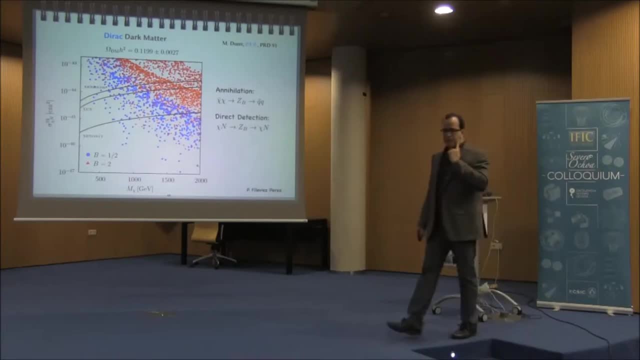 easily. You can actually satisfy the experimental bounds in a nice way Here. you don't need to assume anything. Very peculiar scenario to explain the really density of that matter in the universe And this is always welcome. but again, I didn't think about any that matter. candidate. 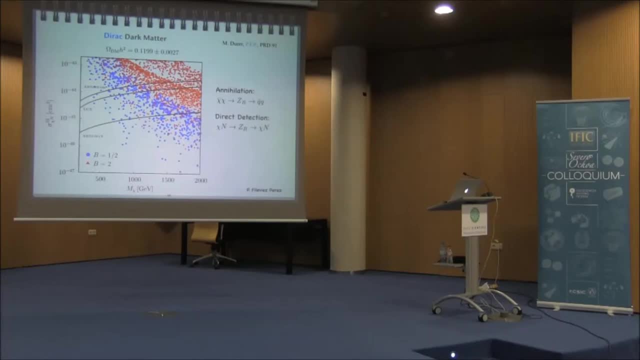 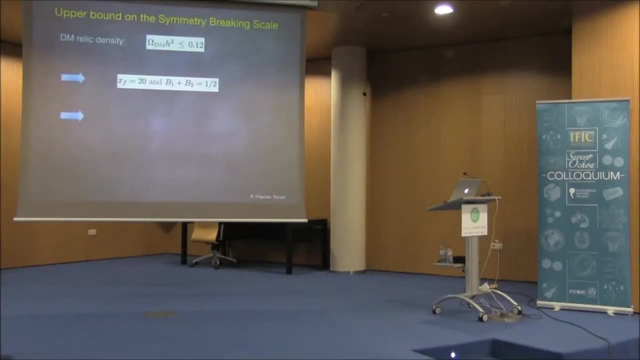 from the beginning. I was looking for something different. This is like a bonus that you get from the theory. okay, Now I told you that I can break this symmetry. I get the proton stability. I have explanation dynamically to explain the proton stability. 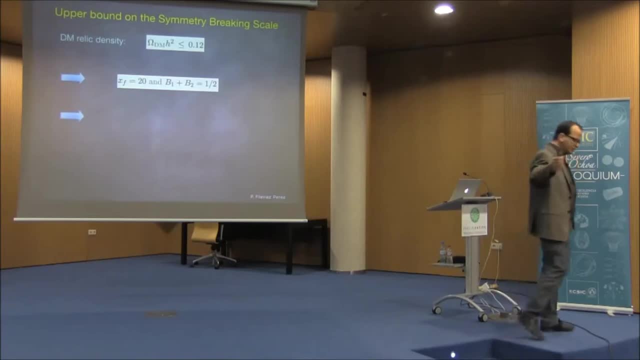 But you can tell me this is very nice, but you know you can do this at the gamma scale, as Georgi Glashow And we never will know about this right, You can do this at any scale. A theory you could do that. 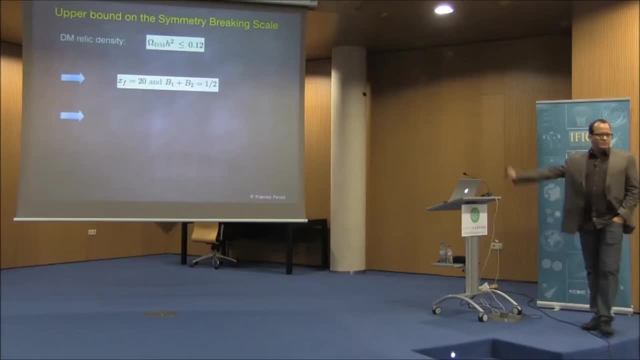 And the LHC, for example, never will see that okay, But the fact that there is a that matter candidate in a theory, you should be a little bit more careful Because there is a limit on the really density of that matter from cosmology. 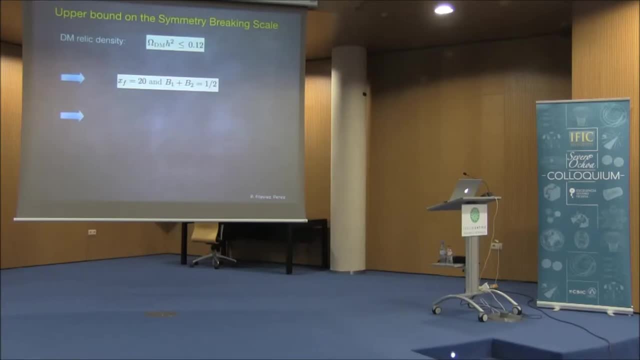 Which is actually pretty impressive. okay, You could say this is even high precision. okay, I didn't write down the error, but this is actually pretty amazing how well we know the bounce on the really density for a that matter called that matter candidate. okay, 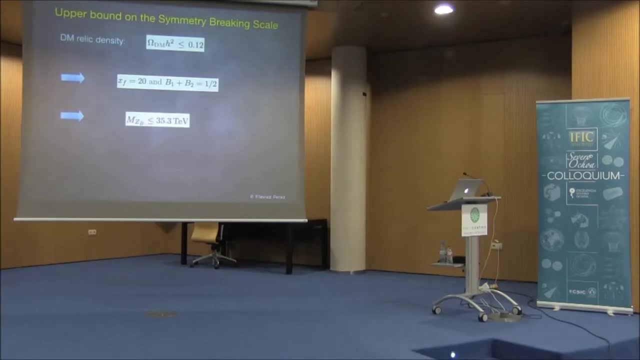 Then if you check this exercise, you'll find that this new gauge boson associated with the breaking of the symmetry, If you want to, If you want to avoid- although we say sometimes over the universe- has to be below some 30 TV. 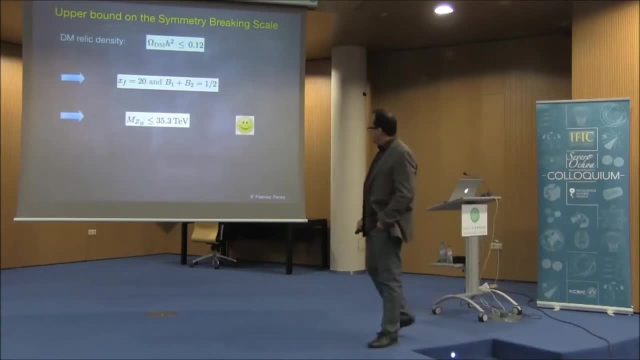 This is like K, And this is good news because you know you smile here. I mean you can smile when I tell you the proton is stable. You have a theory for that Why you have to smile: Because you know the gamma scale I was talking about is 10 to the 15 GB. 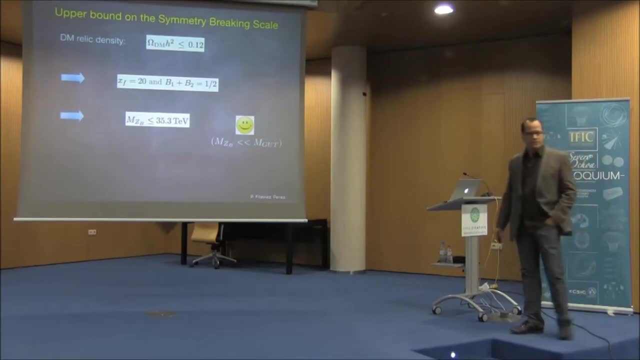 This is just some TV. It means that this symmetry has to be broken at the lowest scale. Okay, Has to be. If you know I am in trouble with cosmology, in the simplest, simplest theory then you get something interesting. If this has to be broken at the lowest scale, then collider experiments could hope to look. 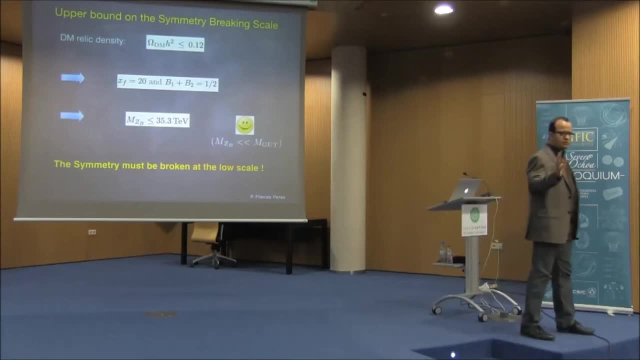 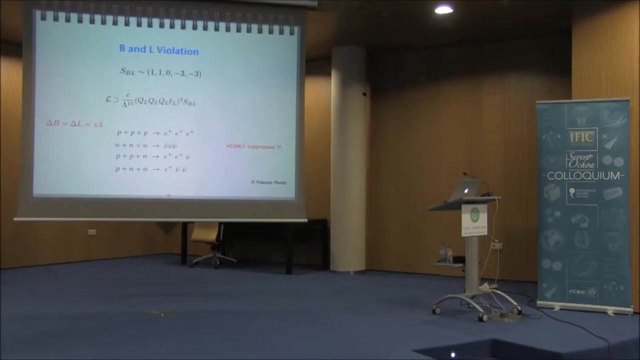 for that and maybe they find something, Because you have a very strong motivation from proton stability and cosmology here to look for that. Okay, If this theory is true, of course, Okay, You can ask me. often people ask me a very exotic process. I will skip that. 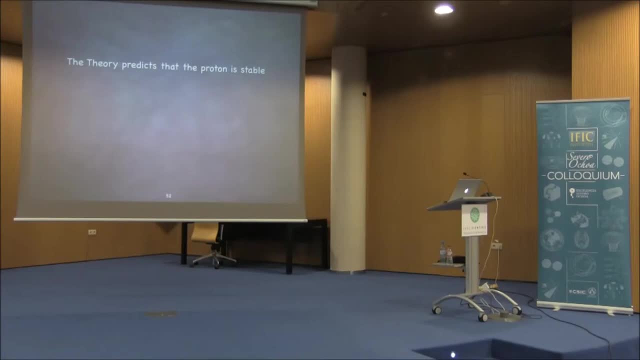 And the important thing here is again the proton. The theory predicts that the proton is stable. This is a very simple question that anybody can ask Any children from. well, maybe, okay, it depends which is the kindergarten, but I guess let's. 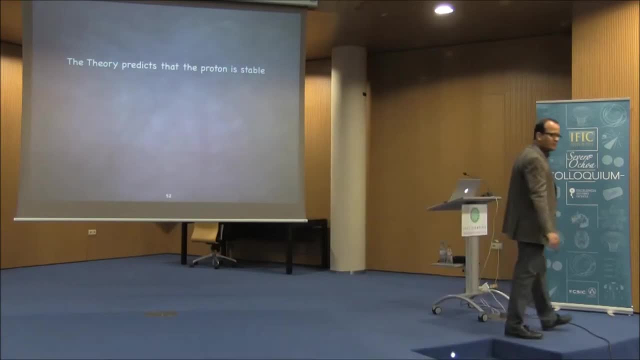 say high school, They can ask you if the proton is stable or not. Okay, Because the neutron decays, but the proton doesn't like decay. Okay, And I told you the whole story started, that George and Glashow wanted to understand the 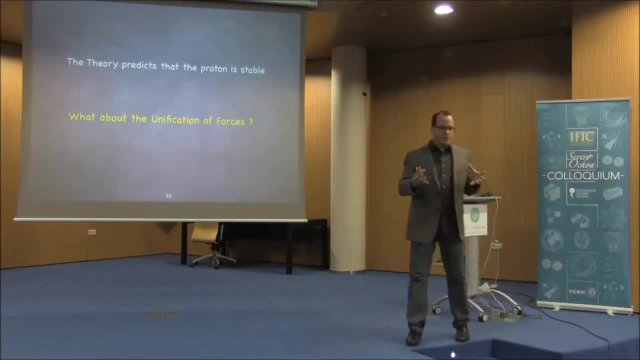 unification of forces, and they had this amazing prediction that the proton has to decay. But here I told you, this theory, where you understand the spontaneous breaking of a bar in number, tells you that the proton has to decay. It tells you that the proton has to be stable. 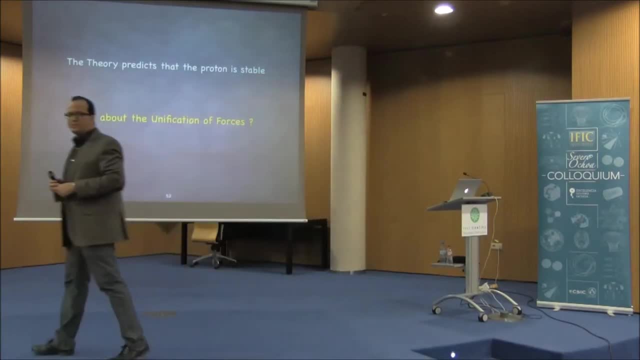 Then, as I told you already, you start dreaming about unification here, Because this you know these lines- that they were meeting at some higher scale. this was consistent because the proton decay bounds are too hard, But now the proton is stable. maybe this meeting can change. 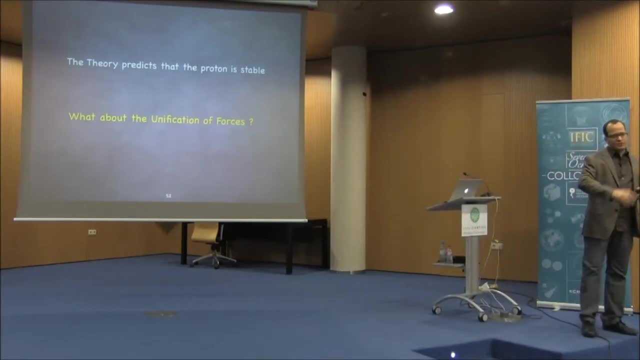 And I can do this at this scale, but maybe the Large Hadron Collider or the next collider could test that. Okay, Okay, Then this is why I say: what about the unification gauge forces? Okay, In this new type of theories. 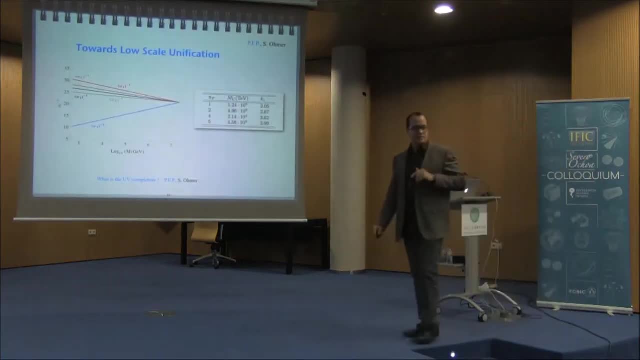 Okay, Well, you can play many games here. Okay, You can play many, many games. The proton is stable. You don't care about the proton anymore. But you can do the same analysis that this guy did in 74.. Okay, 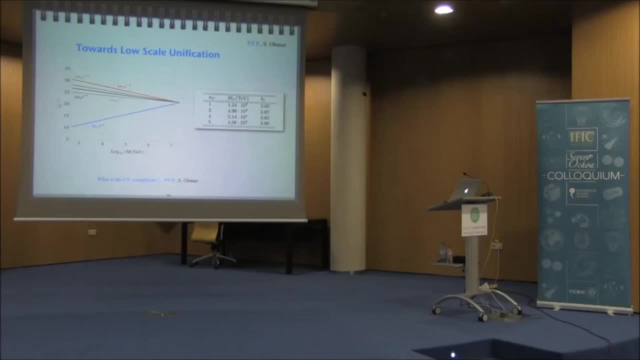 And try to see different scenarios. Here I show one, for example, that the unification is at 10 to the fourth TV. This is the LHC kind of see that If you, you can go beyond that. The only thing that you have to do is you can have new copies of these fields. 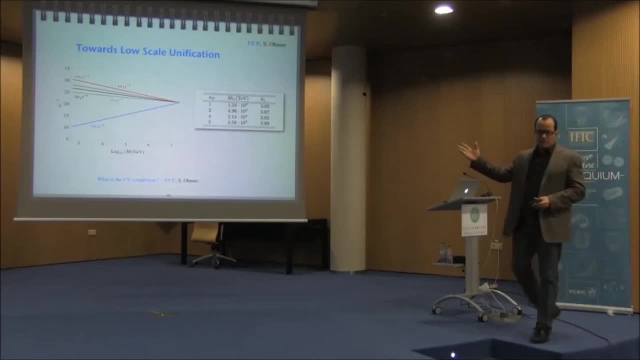 And you can change the evolution of the couplings and maybe you can make a meeting at TV And this is okay because, again, there is no problem in cosmology: The proton is stable. This is possible, Okay, But this is just like a naive exercise to show to the people that this is possible. 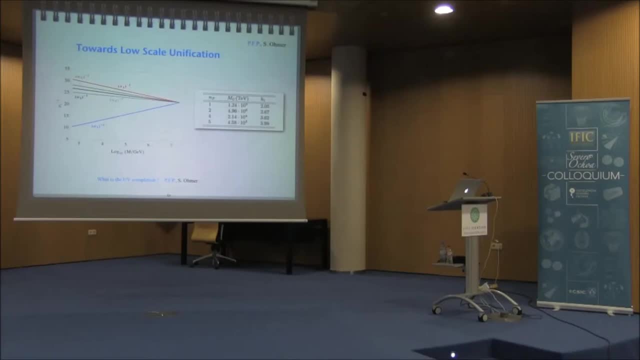 You have to do better than that, Because once you know that Georgie Glashow can do the job, you should do more than that. I have five minutes. Oh yeah, I'm fine, Good, Okay, And then again about this. 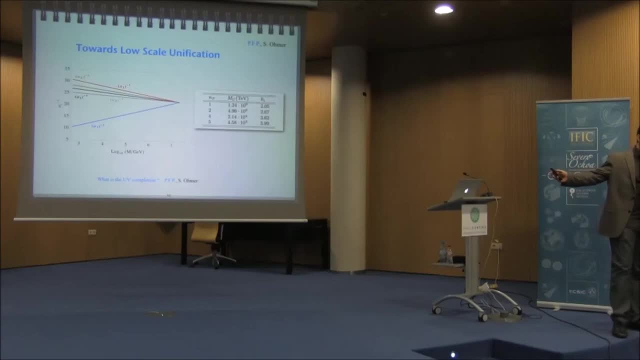 You know, I am already happy enough to be able to say to you: you can write a theory where the spontaneous breaking bar number can explain the stability of the proton. There is a strong connection to cosmology. Cosmology- tell me, be careful. 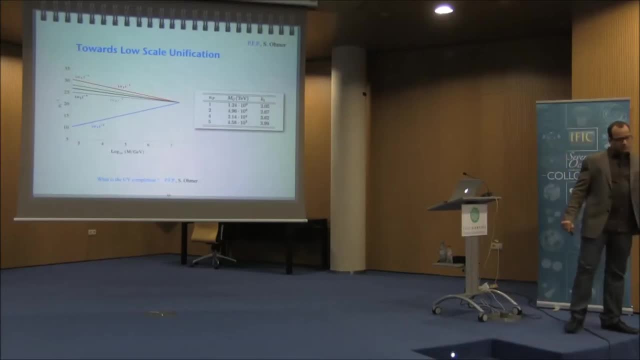 You have to break this at the lowest scale if you don't want to overclose the universe, if you don't want to have too much. But of course you want to go back and try to reproduce the same thing that Georgie Glashow did. 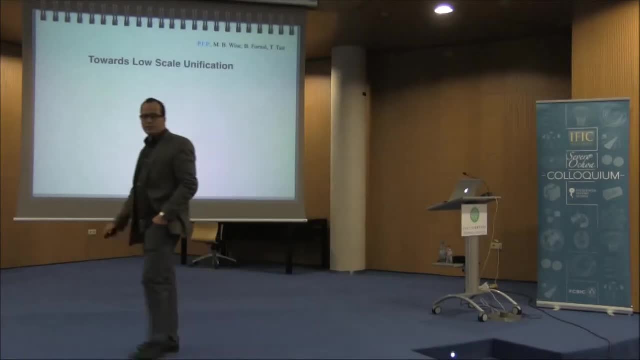 Okay, But I told you, sometimes people don't like to live together In the usual grand unified theory. again now you want to say, okay, in the usual scenario, I have S of 5. They never will know about this because the scale is too high. 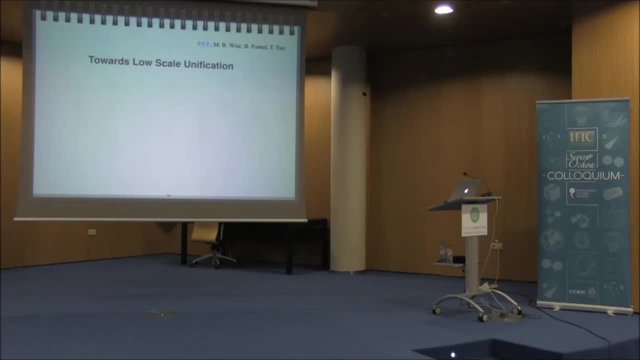 Never will know about this. There is no way to know about this, But it's very pretty, Just S of 5.. Okay, And then I told you: this is like the theory that you have to have, let's say, the TV. 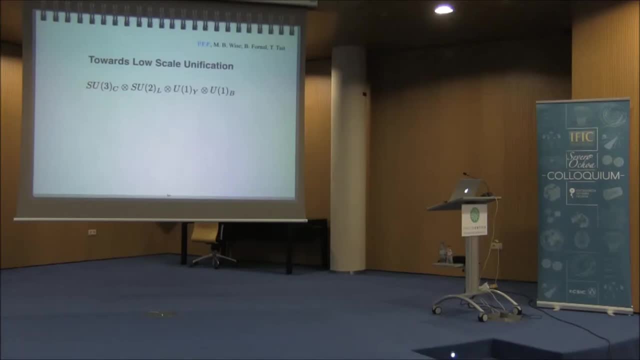 scale here And it will be nice to unify that in a very simple group. Okay, I personally struggle like crazy thinking about it. You know, I guess I hope to find something better When I will show you I still not happy about. 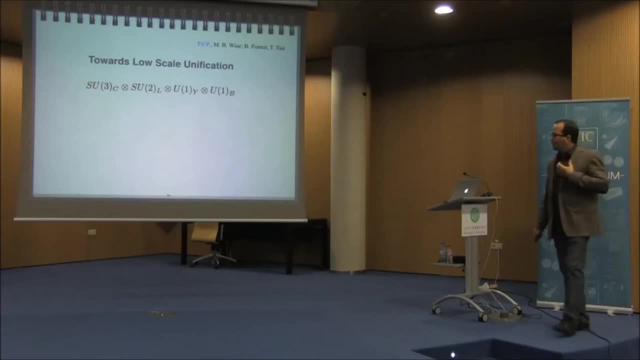 But you know, This is how you do science. You try, Okay, And then the key idea is actually pretty simple: The quarks, they feel the strong interaction and they have barrier number. Then it's natural to assume, okay, this is QCD and this is the barrier number. 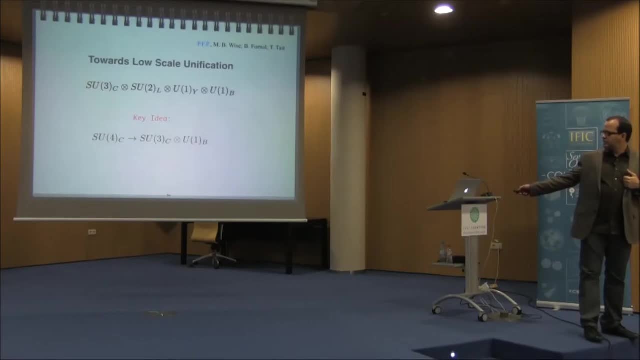 It's natural to assume that you can unify these two guys in S of 4.. In a new symmetry that is called S of 4 color Okay, Because they are only the quarks have this property. The electrons they don't have barrier number. 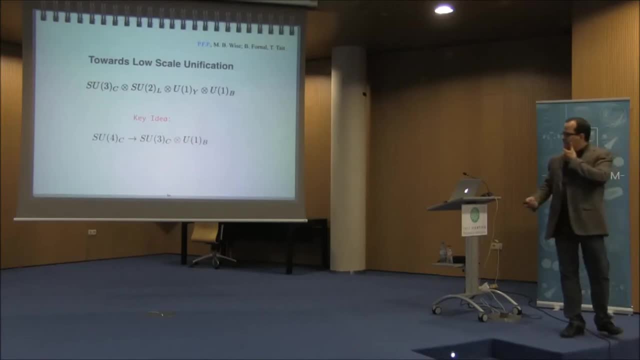 And they don't feel the strong interaction. You cannot do that, Okay. This means that you have to unify the quarks. They understand the model And then you can imagine that you could have S of 4 color, S of 2 left, U1, hyper-sharp. 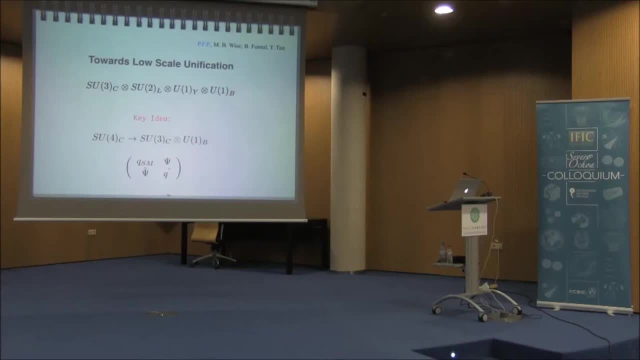 Okay, Unify strong interaction with barrier number, Because barrier number is a local symmetry. It's like a new fundamental interaction. Okay, And then you can do, you can try more, You can try harder, And the best thing that I find, 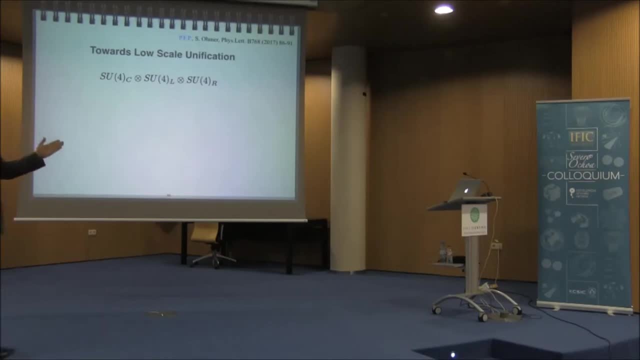 So far Is that you can unify everything in S of 4 cube, Okay, Instead of having S of 5.. That is very simple, Very nice, And so The best so far that I found that is- This is the previous theory. 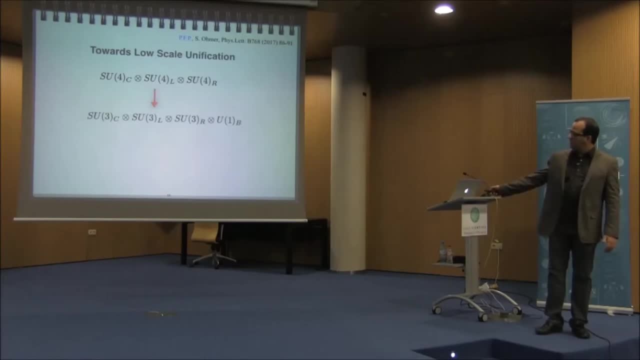 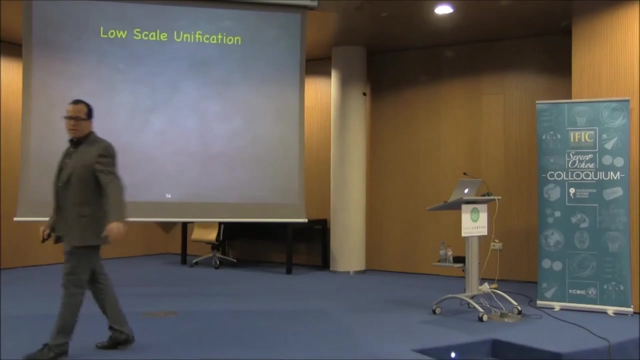 That you can break to something that is very well known to unification With barrier number And when you break you get this theory that I mentioned that has to live at the TV scale. Okay, But maybe you don't like this theory. I don't even care about this particular example. 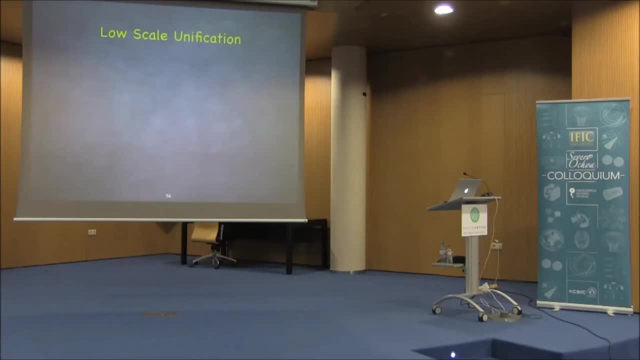 I think the idea is so generic That anybody can take this idea And try to build something better. Maybe string theory is true, I don't know- And they can have embedding a more fundamental theory together with gravity, I don't even. 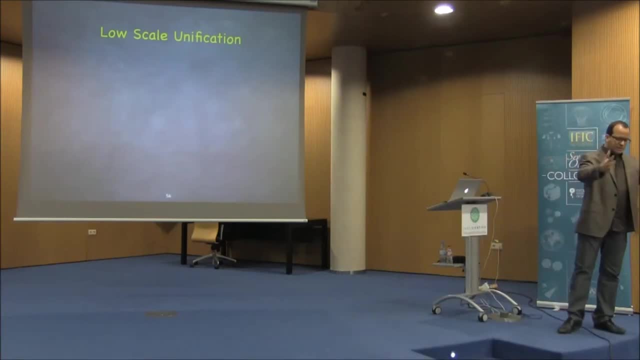 You know This is just a possibility, But I find this so appealing that I can explain. the proton stability Cosmology tell me that I have to do at the lowest scale And means that the collider People can actually look for that. 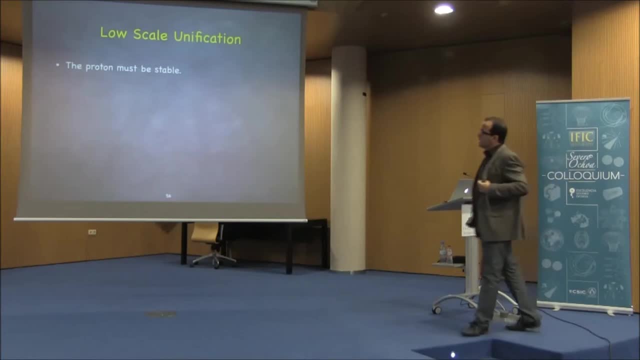 Okay, Then the lowest scale unification again means that If you don't try what I said, I am afraid that the only way to explain the proton stability In a fundamental way is this way. I don't see a different way. But again, if you want to unify, 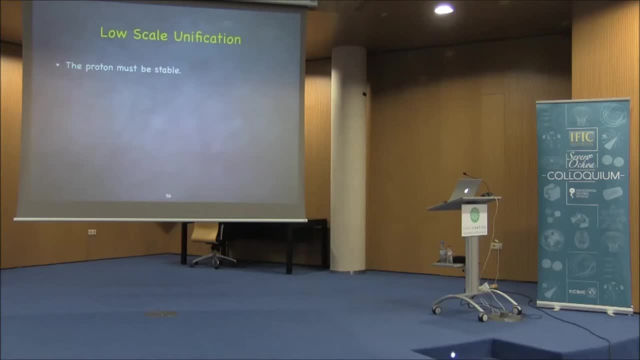 And change the rules of unification forces At the lowest scale. Again, the proton has to be stable, Of course. You have to do this at the lowest scale And you suffer Because you don't have a sulfide. that is so pretty and so simple. 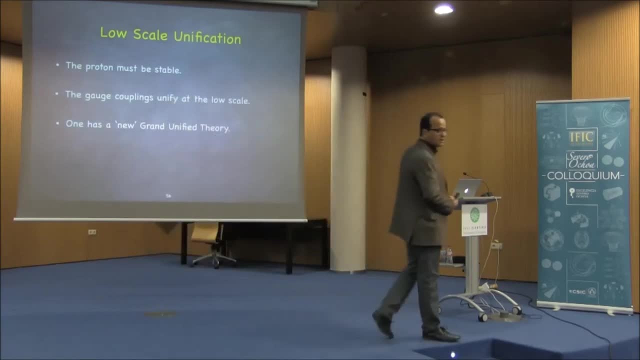 You have to find a unified theory. If there is a unified theory like that, Which is more involved, Okay, But the idea again is very simple: Proton stability. Then you can go to the lowest scale. Okay, Then In this way, 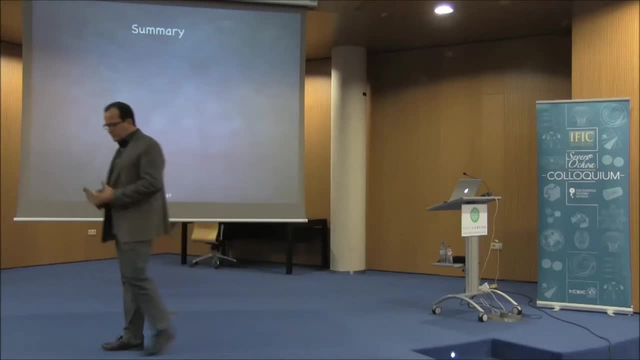 I will summarize For people that are no experts, For students. You don't have to remember Any of these things. I only want to tell you a few things. I told you that in the usual, Using the usual idea of grand unified theory, 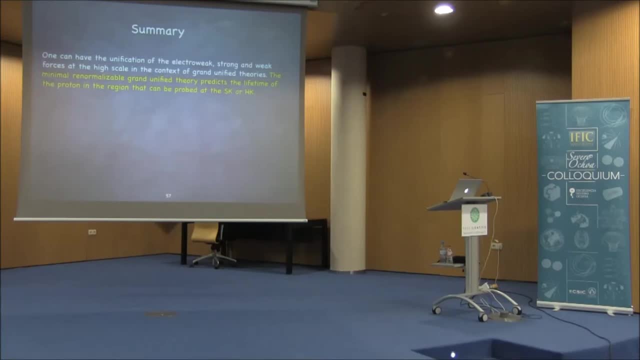 Which are very, very, very appealing. You can understand the unification of the strong, Weak and the electromagnetic interaction, But this happens at the very high scale And maybe You can see proton decay one day. Maybe, But you never can make a test of this idea. 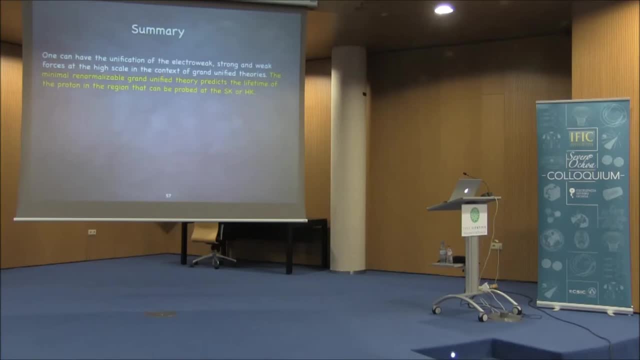 Never, Because we never can have access to this scale. Direct access, Okay, And I told you there is a different way. If you write a theory for a spontaneous breaking of bar number, It means that the bar number has to be a local symmetry. 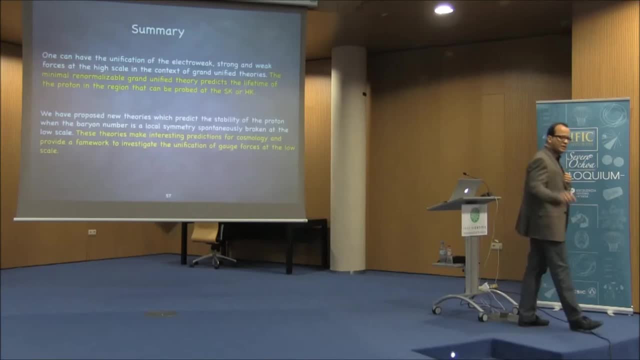 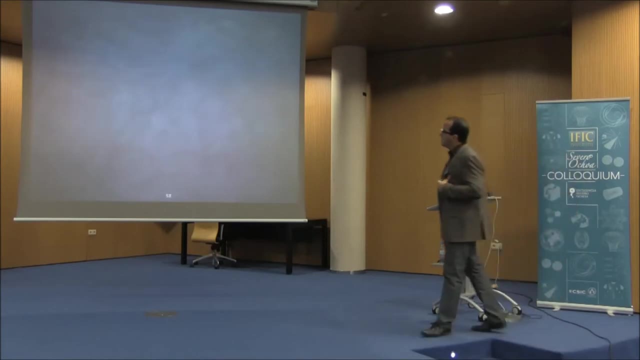 You do a spontaneous symmetry breaking of that, Here you find. Here you find that the proton is stable, Then you can change all the rules of the game. Okay, Then, To finish, There are two Pictures that you have to use. 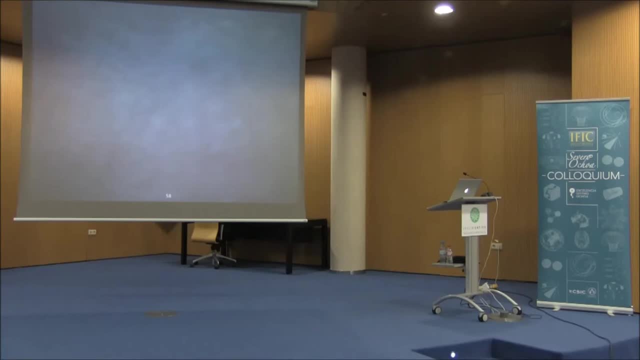 Okay, Maybe, Maybe Our understanding of fundamental forces, Or the unification of forces, Is like that. You know this Weird thing that you have two big scales, Two scales that are far away from each other, Or maybe, Or maybe. 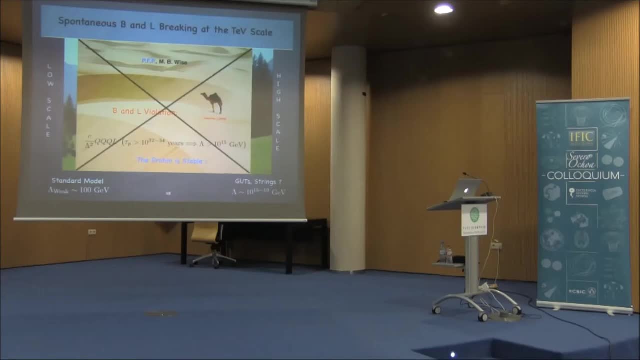 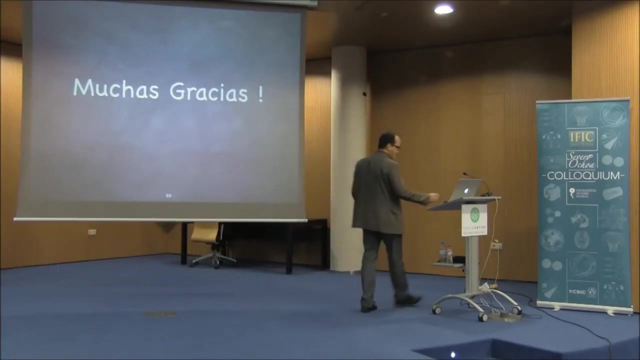 It's something like that. You don't need that. The bar number is a fundamental symmetry in nature. It's spontaneous, broken The lower scale And things can be different. Okay, Muchas gracias. So thank you very much for this nice overview. 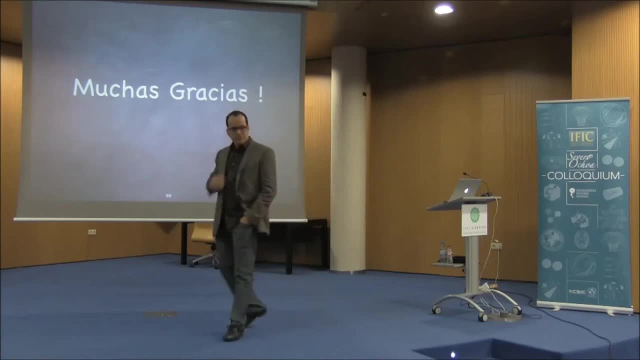 And now we have time for questions. I apologize if I was maybe a bit too technical sometimes, But if you have any questions I'd love to Paul, Could you comment a bit on the barium asymmetry? Okay, I don't have a slide here. 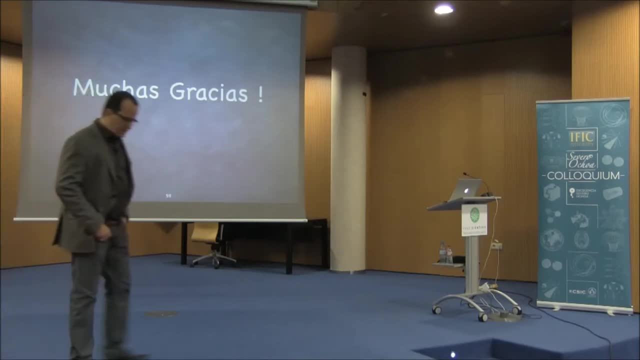 But this is actually a very, very good question. When I started thinking about that, The people told me that I was dreaming, Because I never would be able to explain the barium symmetry, Because they are so-called Sahara conditions, One of the Sahara conditions. 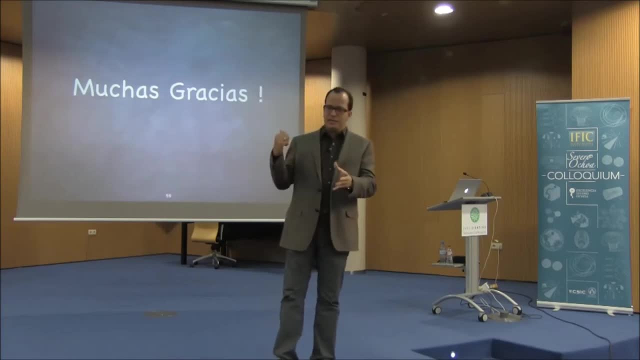 Is that you have to break barium number, And here I am very radical, Even when want to break at the very lowest scale, and the experiment allowed me to do that. However, what happens is that what I did was, you know, there is a very well standard. 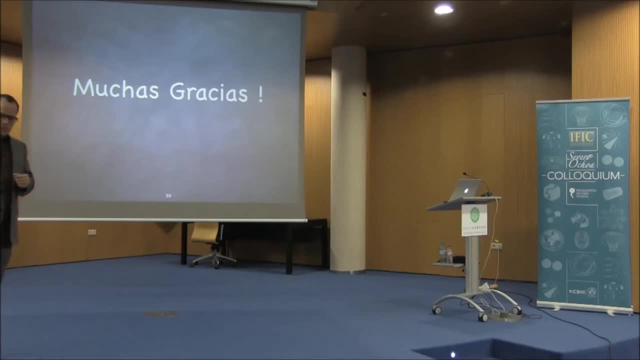 analysis is that you take the whole standard model, you assign a chemical potential to all the fields in the theory and you do the temerary equilibrium equation to solve for that and you find that the usual thing is that they are as far in the process that they. 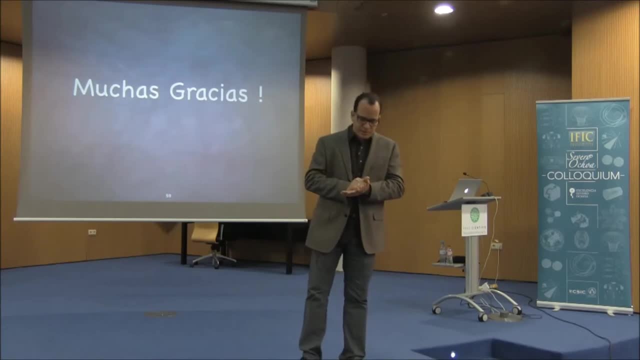 convert any B-minus cell asymmetry and generate the baryon symmetry. Here what happens is that we manage to find that if the symmetry is broken at the very lowest scale, the sphagnum conditions are different, and I can write down that the baryon 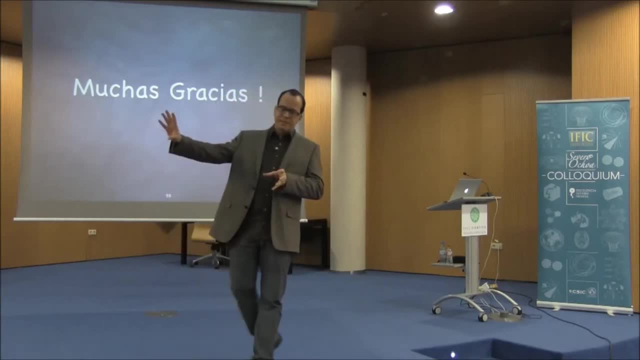 asymmetry is a linear combination of the B-minus cell asymmetry plus asymmetry in the Darmadal set And you could have something that is called asymmetric Darmadal, that you have a relation between asymmetry in the Darmadal set to connectivity. 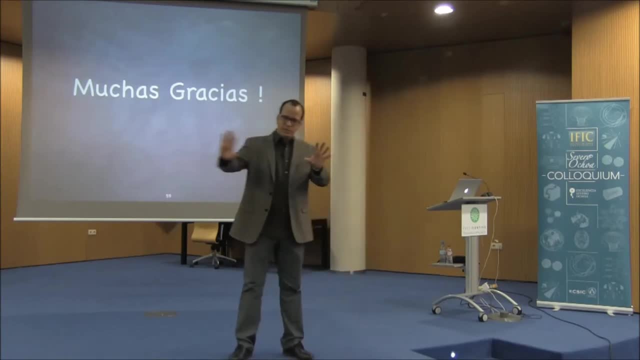 Or if there is no this asymmetry I will have, you find that the sphagnums they do the sensing, but the coefficient that we call the conversion factor is a little bit larger. But you can find a consistent relation between baryon symmetry, B-minus cell asymmetry and 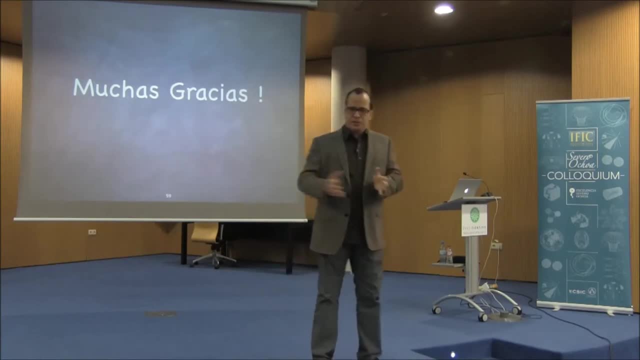 Darmadal symmetry without having any fine tuning in any chemical potential in the theory, And this is how it works Without Without giving any major detail. you have to think that this is maybe a box and this box has two parts. One is that these new fields that are there for anomaly cancellation and the standard. 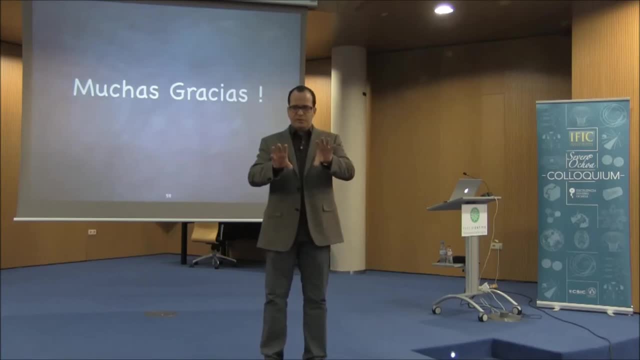 model here And there is a baryon number violation in the standard model and a baryon number violation in this new set. But the total baryon number is conserved And this is a consistent way to see why in our set we see a baryon symmetry. 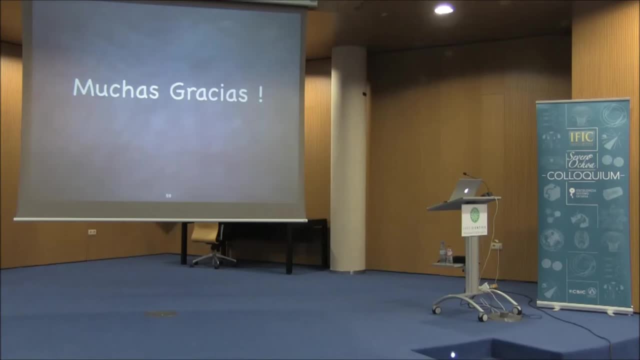 More questions. Okay, The fundamental difference between your theory and every other theory is that the proton has to be exactly stable, right? So we have super K, that says 10 to the 34 years. hyper K is probably 10 to the 35.. 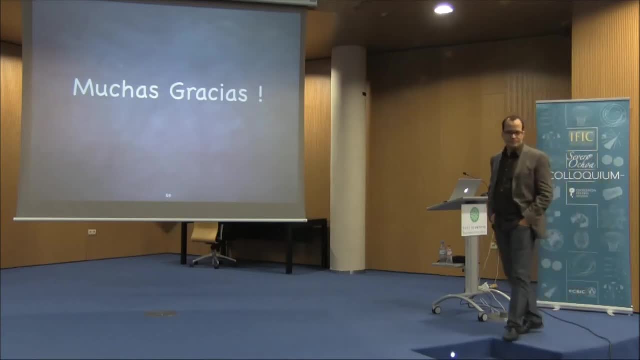 How many, How much larger would you have to make That experiment if you want to really answer the question whether it's stable or just long-lived? You know, before I was born, they started to think about building these detectors. okay, 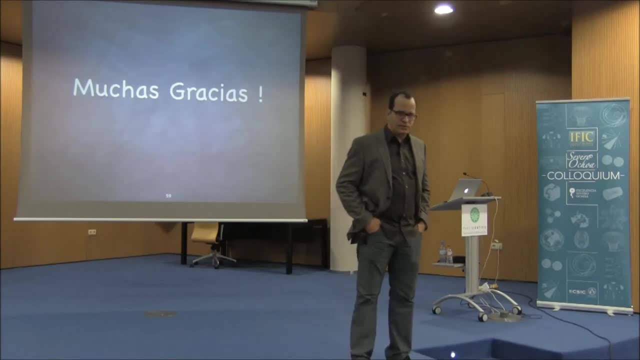 Then the honest answer is: maybe the usual idea of granulofyte theories are true, But in reality I spent a lot of time working on granulofyte theory and proton decay and it's You try very hard And the honest answer is: you never can make a very high prediction for proton decay lifetime. 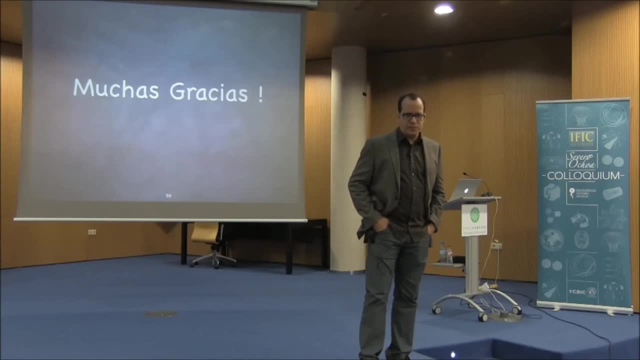 Nobody knows. If the proton is not stable, nobody really knows. You know, you're reading many places- that will dictate tomorrow and you will say tomorrow, because the theory supersymmetry or any theory that somebody said is beautiful, predict 10 to the 34.1.. 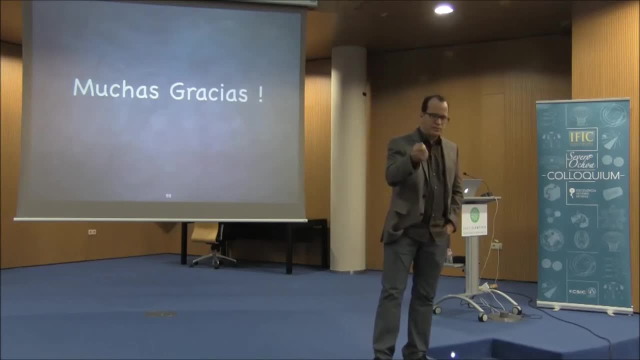 But this is Nobody really knows. When you really do the whole calculation using kind of perturbation theory or all the models element and you do the best calculation for the catascale, it's depressing, It's very hard. Nobody knows. 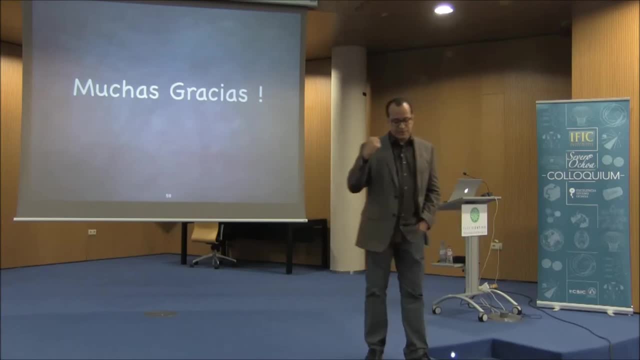 And the other possibility is that the theory is stable. That means that it's good that super K saw neutrino oscillations, because if this is true, hmm, better not to have so many photon multipliers to look for proton decay. But they did a lot of science with neutrino physics, which was pretty amazing. 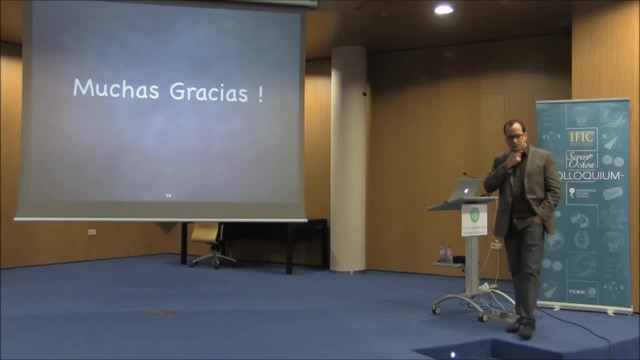 Yeah, If I want to scale up. Yeah, I want to go to really answering the question: is it stable or just long lived? I guess if the gut scale approaches the proton scale at some point I'd become convinced that it's down. 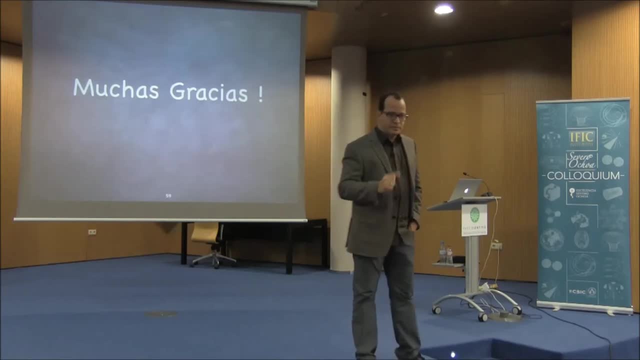 It's more simple than that. If you find at the collider this gauge, bosons and so on, you put, you take score of this field and you realize that the baron number was broken three units, you're done, Because the proton never will decay. 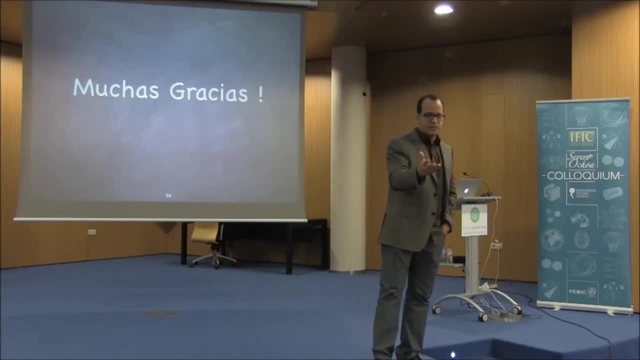 I know, Of course, this is the first answer that you can say, And this will give you a hint: okay, looks like it doesn't want to decay. This is the best thing that you can do: Score these at the colliders and make sure that you understand that it's broken. three. 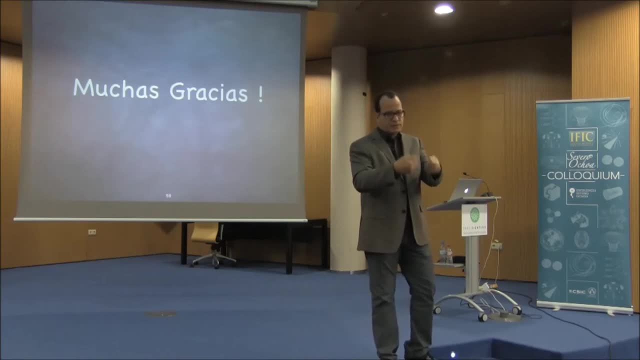 units, baron number. That means that proton, in this context, never decay. But it's hard to go beyond that. That will happen, probably not at the LHC, We don't know, We can't. Depends on the mass. Depends on the mass of this. 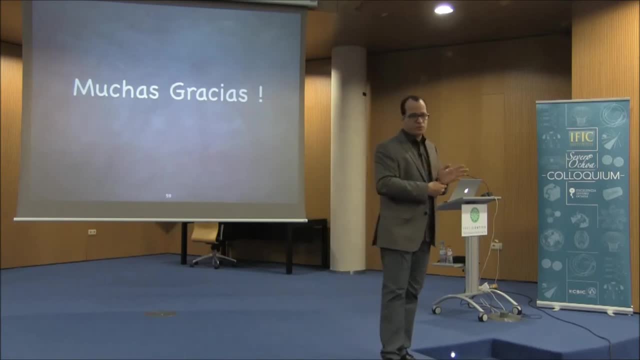 I am not able to predict. I'm only able to use probability, I'm only able to use cosmology to put the upper bound on that. It's very hard. You can have three units decay. Yeah, okay, thank you for asking this question. 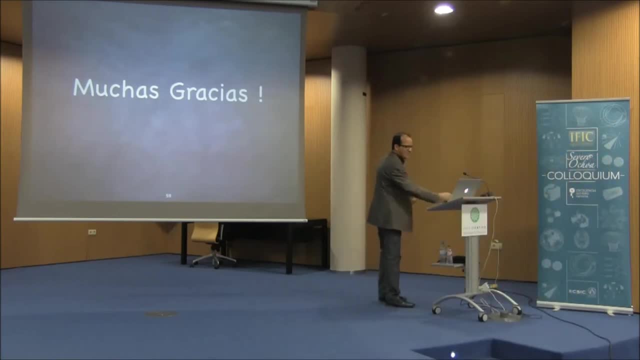 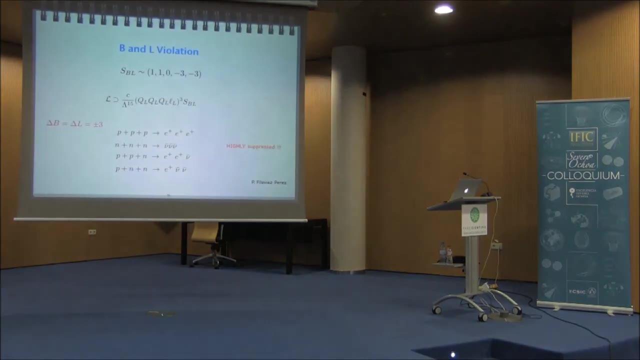 This is one slide that I didn't show. Thank you for asking this. Now I can go back and show you that, Yeah, This is the three unit decay. You see, you have to be careful because the three units is stable, Okay. 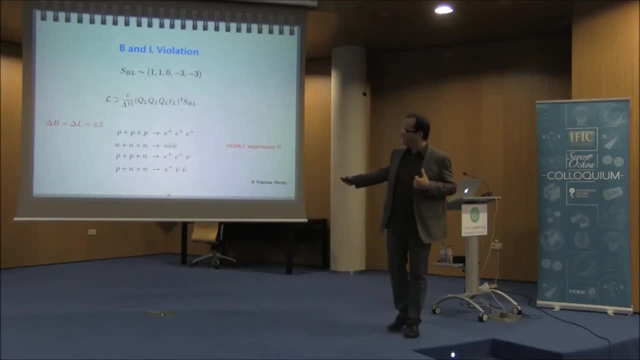 But the point is that if you check which is stable, Okay, If you check which operator gives you three units decay, It's not stable, It's dimension 19. Then, even if lambda is a little weak, this is 10 to the 100 years. then you're fine. 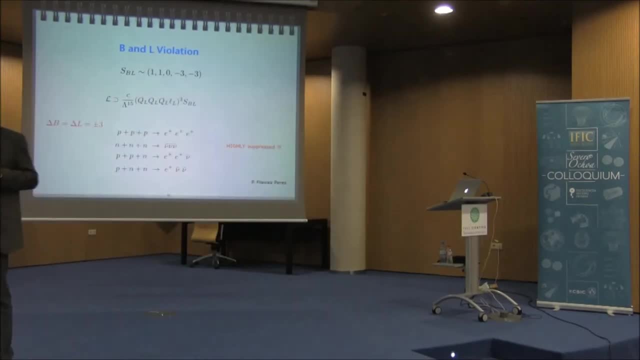 You don't. you are not in trouble with any delta B equal 3 process. You are safe. You are lucky, because this is a really good question- You do this. you will be in trouble with three units decay. The theory tells you that this is highly, highly suppressed.